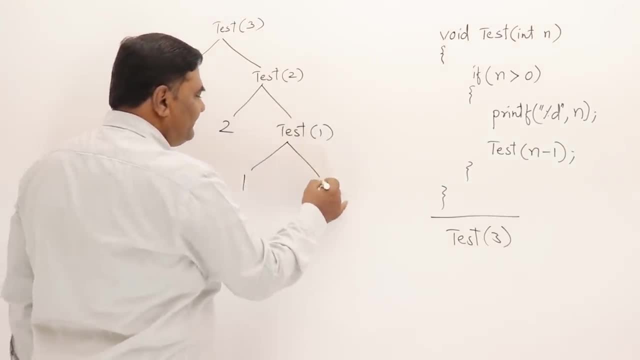 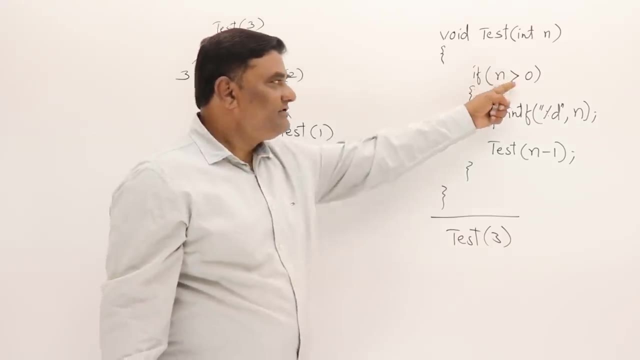 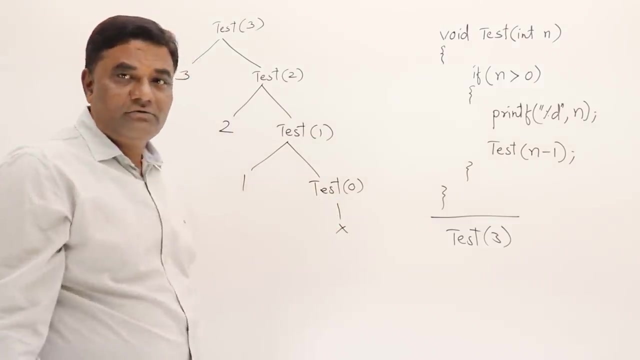 than 0, it will print 1 and call itself for test 0. now, when it is 0, 0 is not greater than 0, so it will not call itself and it will stop. doesn't go further. so this is a tracing tree for this particular function or recursive. 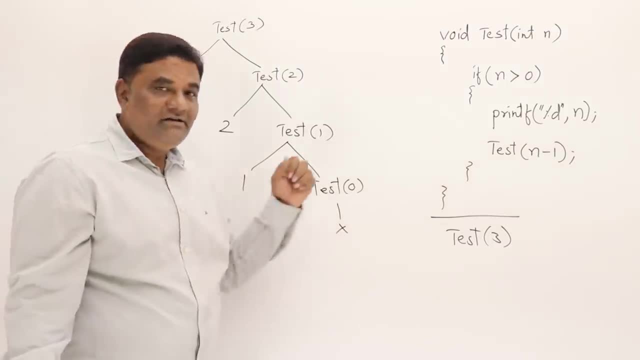 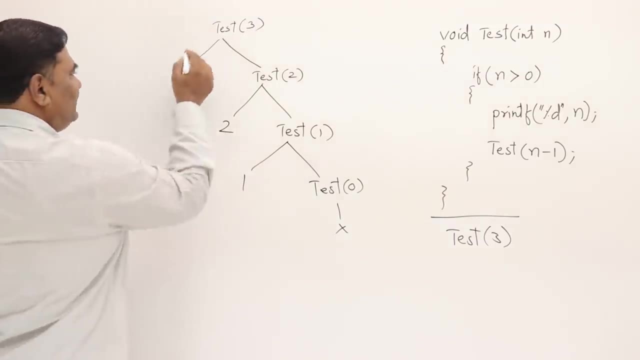 function. I have passed 3, so what is the time taken by this one? so let us see what it is doing in this call. it is printing a value, then calling again, printing a value and calling again, printing a value and calling again. so the amount of work done is just printing value. how many times it is printing? this is the. 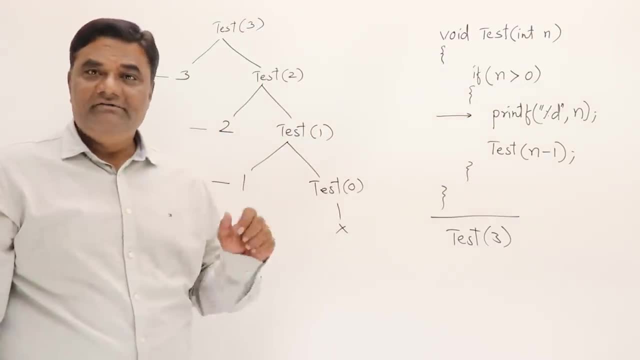 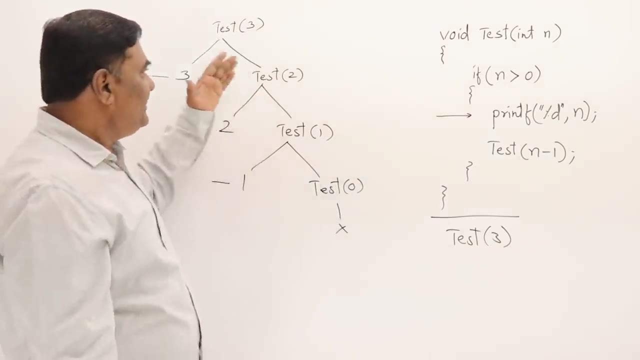 major work done by this function: printing a value. how many times it is doing three times it is doing as I have passed of 3. how how many times it is calling itself as I have given 3, it drawing itself for four times. now, what is the time taken for print? 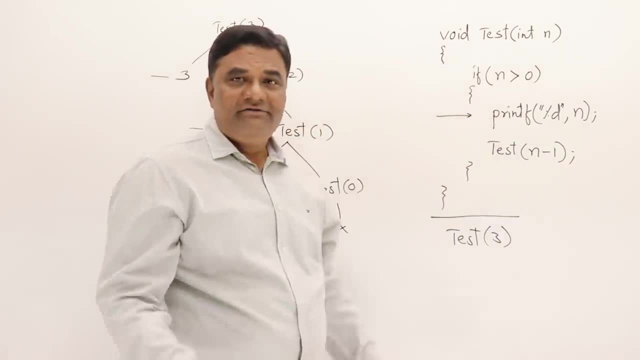 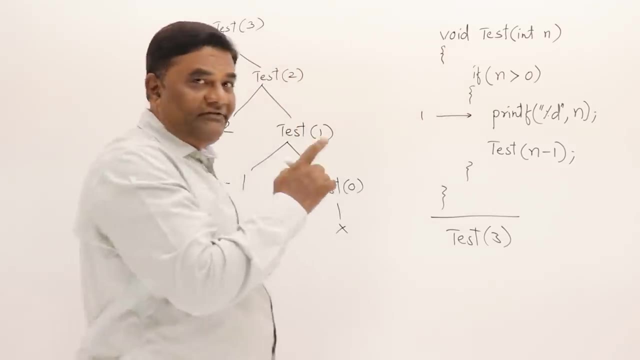 �֗ف. it is just one unit of time. just it is single statement, a simple unity of time. just it is single statement, a simple statement that is taking one unit of time. if I say one unit of time, then in each call it is printing one unit of time. that is printing and then calling. so one unit of. 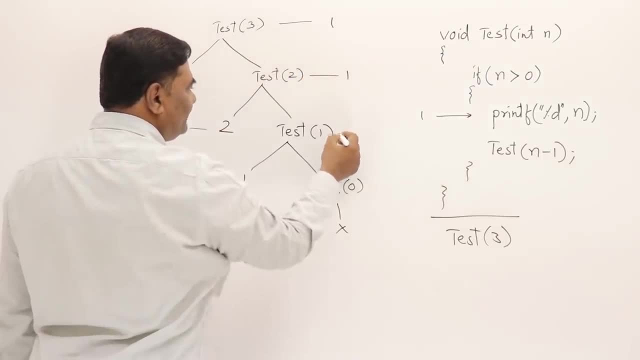 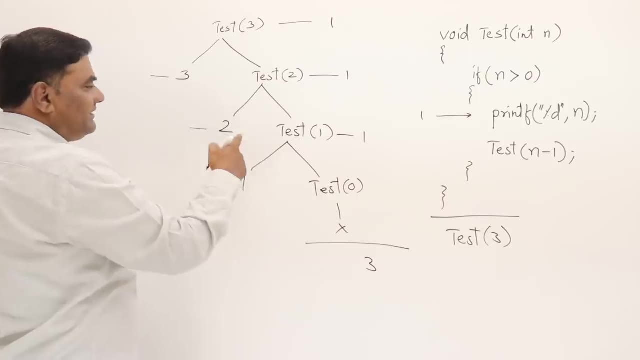 time. one unit of time is capital twins of time, so total how much time it has taken. 3. if I take number of calls, then there are 4. that is 3 plus 1. it means if I pass 5 then it will be 5 plus 1 calls. 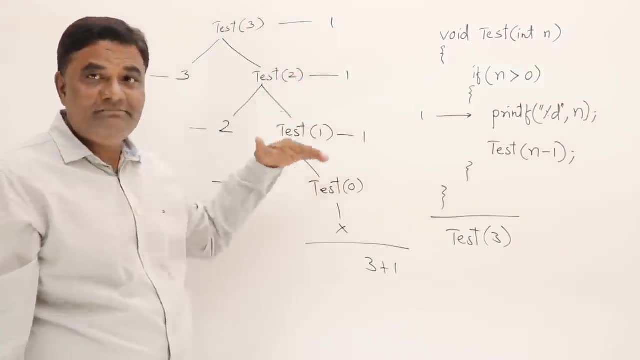 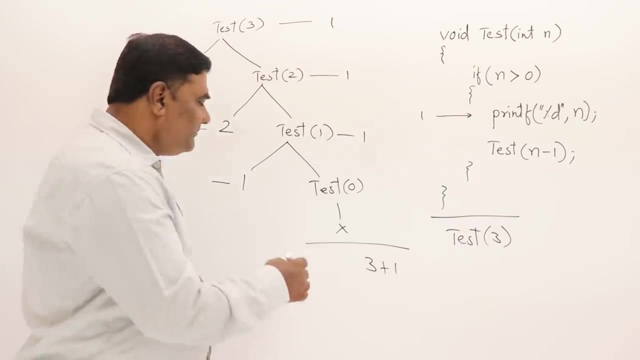 and 5 is the number of time it will print. so if I pass n, then total how many calls it will make. it will make n plus 1 calls, n plus 1 calls and how many times printf is executed- n times if I approximate the amount of work done. 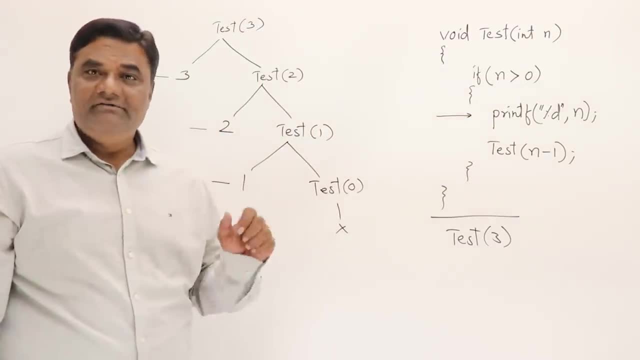 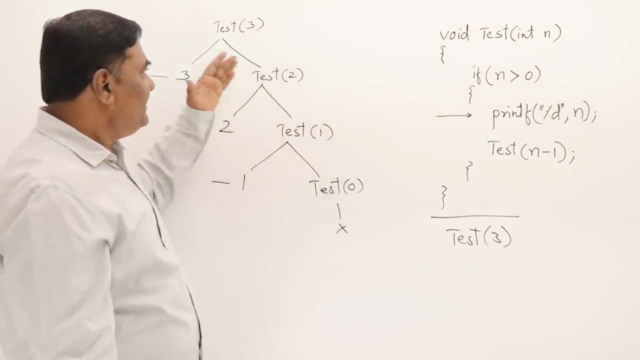 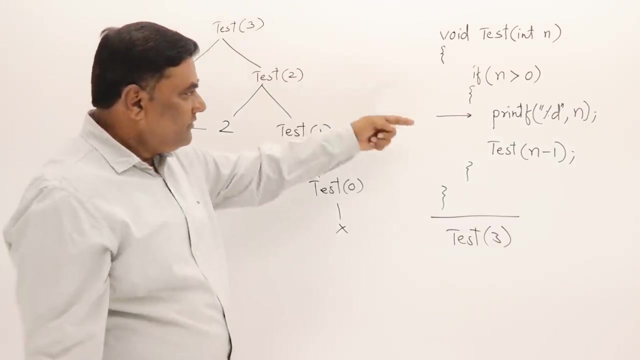 major work done by this function: printing a value. how many times it is doing? 3 times it is doing as I have passed 3. how many times it is calling itself as I have given 3. it is calling itself for four times. now, what is the time taken for print F? it is. 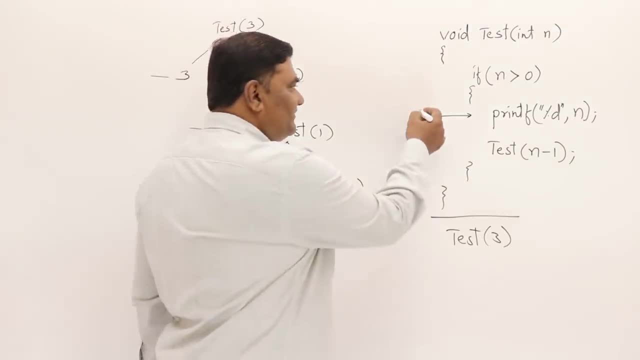 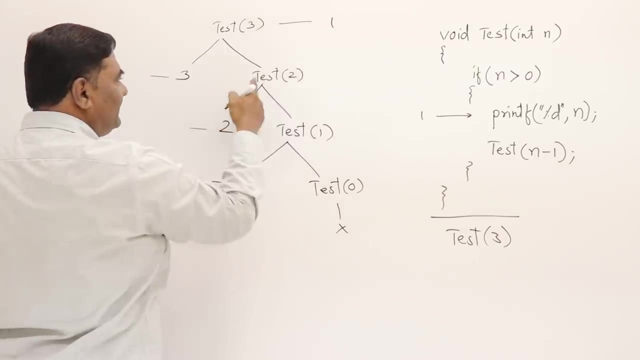 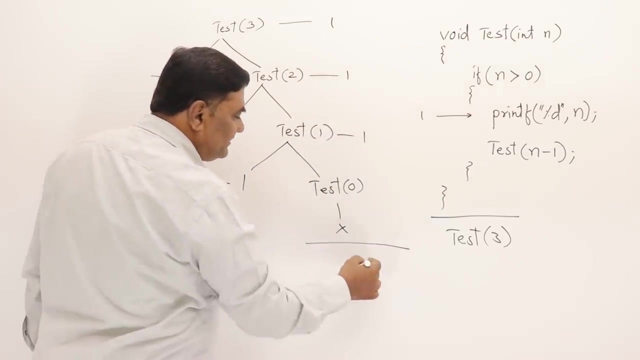 just one unit of time, just. it is a single statement and simple statement. it is taking one unit of time. if I say one unit of time, then in each call it is spending one unit of time. that is, printing and then calling. so one unit of one unit of time, So total how much time it has taken. 3. If I take number of calls, then 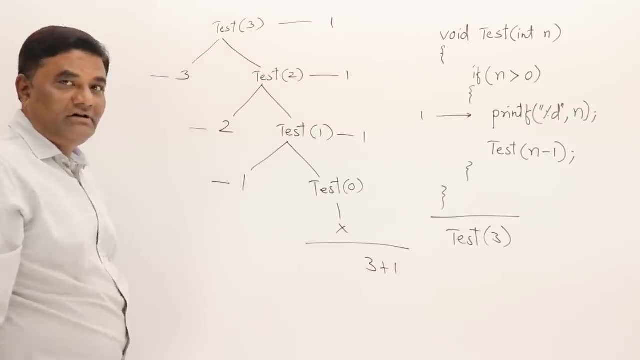 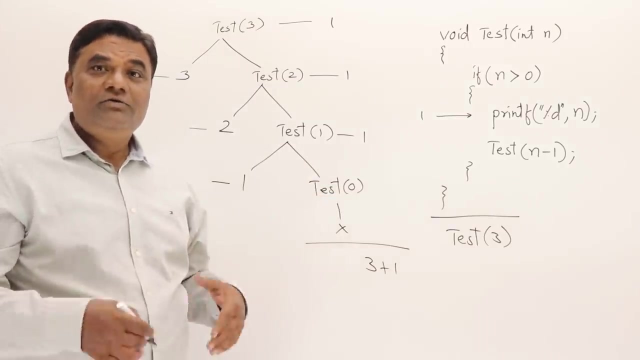 there are 4, that is 3 plus 1.. It means if I pass 5 then it will be 5 plus 1 calls and 5 is the number of time it will print. So if I pass n, then total how many calls it will. 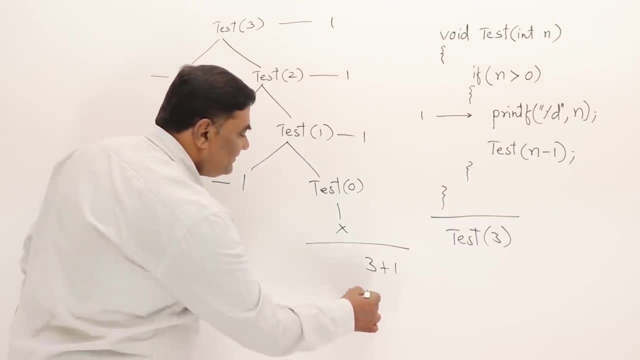 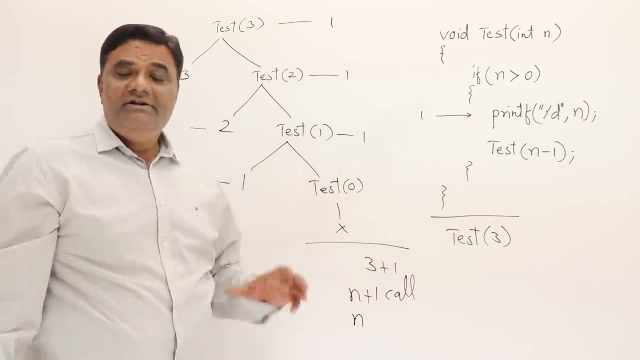 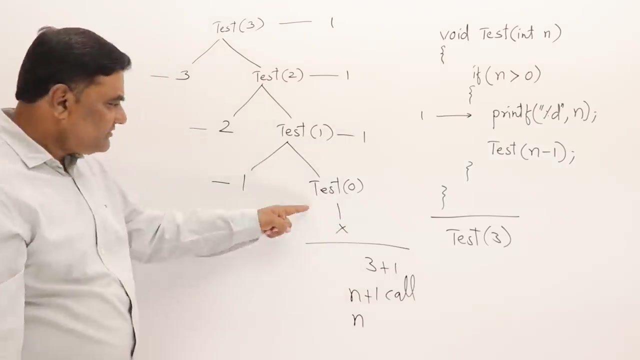 make. It will make n plus 1 calls. and how many times printf is executed? n times If I approximate the amount of work done depends on the number of calls. if I say Like in the last call it is not printing, just ignore that and say that for every call it is printing. 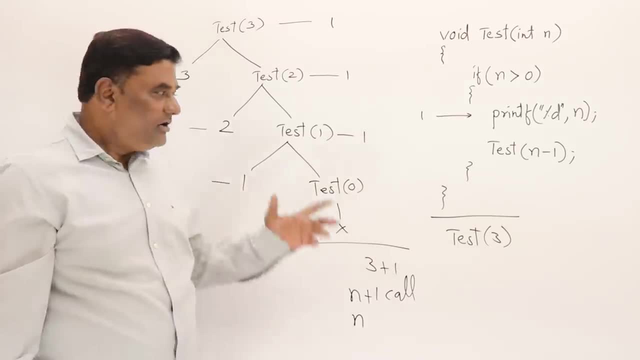 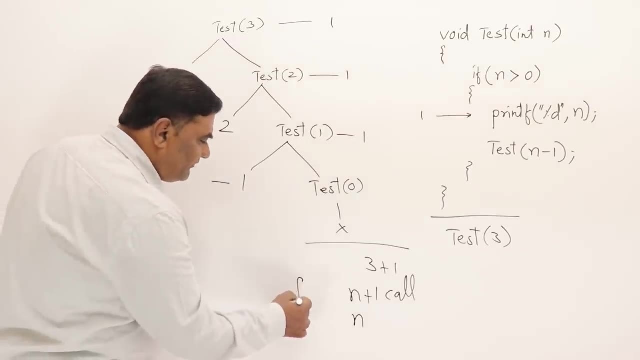 So the time depends on what? It depends on the number of calls. So how many calls it will make for any n, It will make n plus 1 calls. So the time function if I write f of n, then it is n plus 1.. Then what is the time complexity? 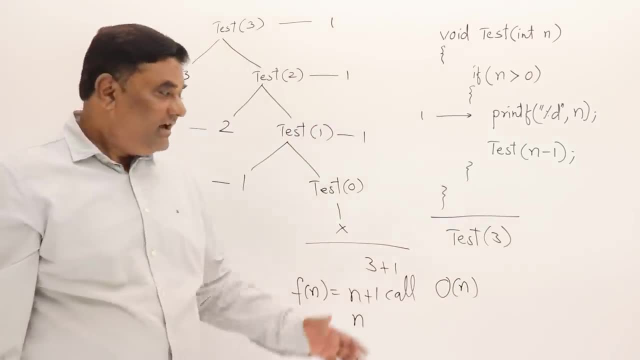 in notations It is order of n. I can use big O of n, theta of n or omega of n, Anything I can write there. This we have already discussed in previous videos. So that's it. By a tracing tree I have found the time complexity of this one. 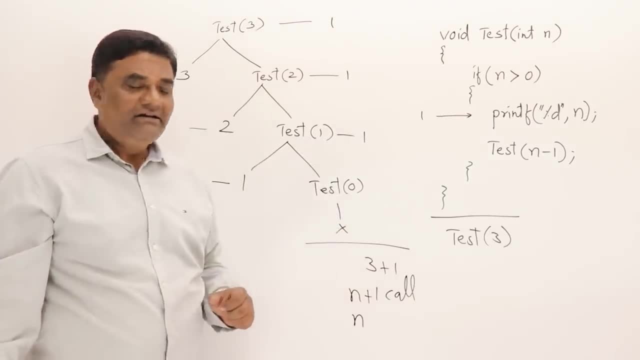 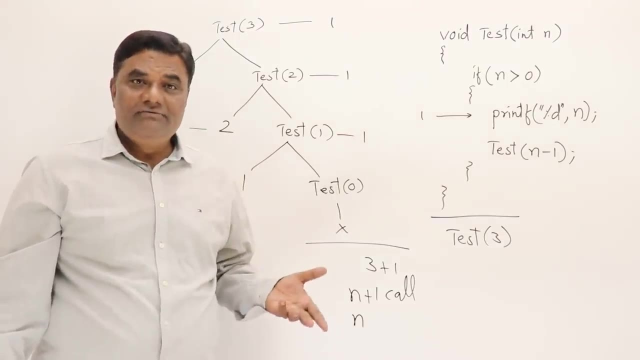 depends on the number of calls. if I say, like in the last call, it is not printing, just ignore that and say that for every call it is printing. so the time depends on what. it depends on the number of calls, so how many calls it will make for. 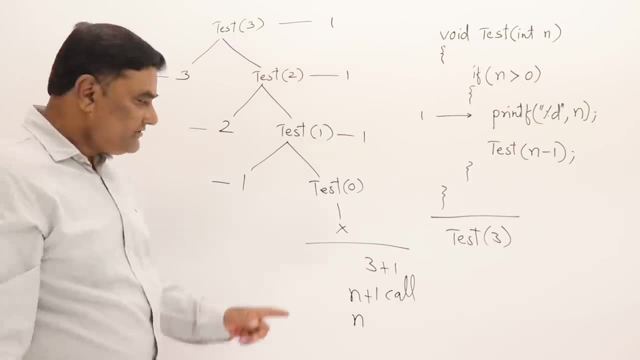 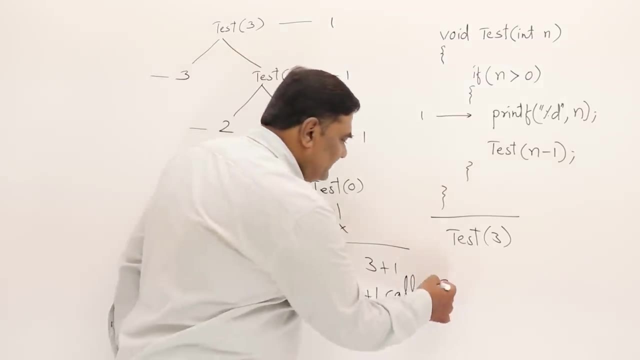 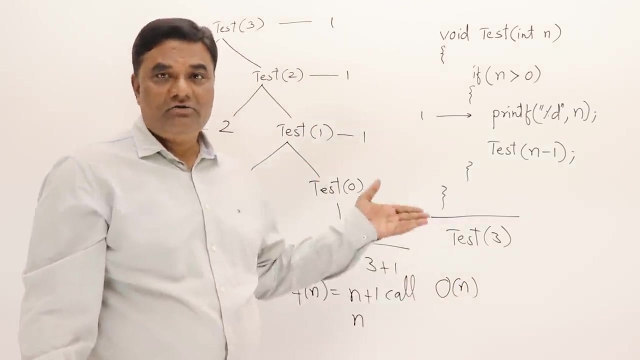 any n it will make n plus 1. calls so the time function. if I write f of n, then it is n plus 1. then what is the time complexity in notations its order of n. I can use big O of n, theta of n or omega of n, anything I can write there. this we have already discussed in. 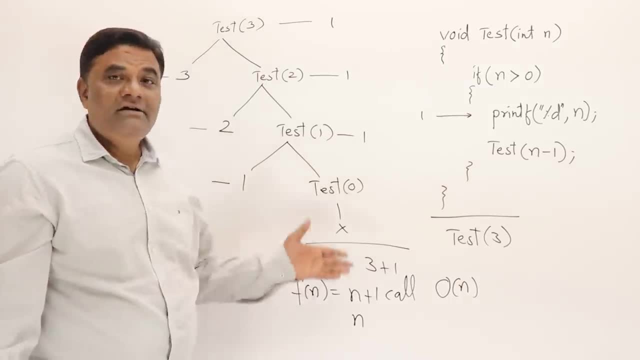 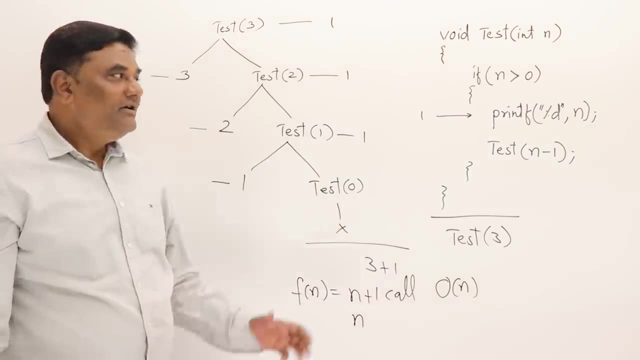 previous videos. so that's it. by a tracing tree I have found the time complexity of this one. you can also call it as a recursive tree or a tracing tree, or a recursive tree I have used. now let us find out how to prepare a recurrence relation for. 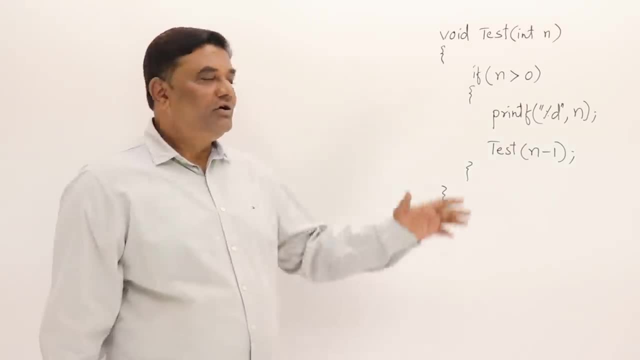 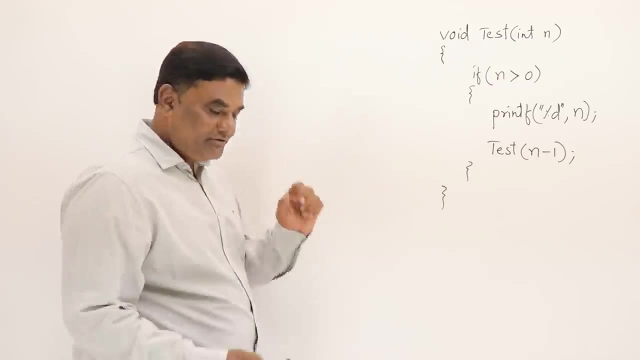 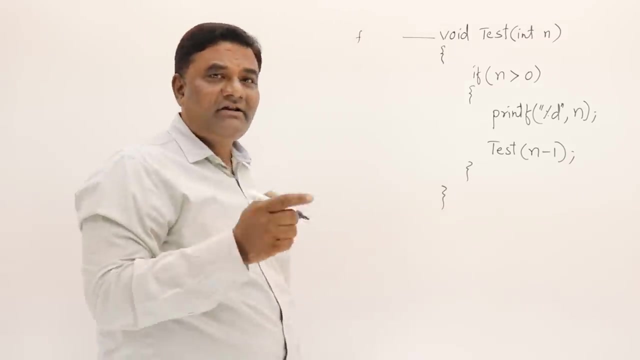 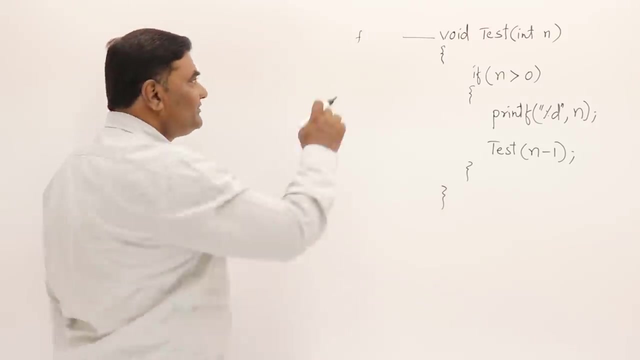 this function and how to solve that recurrence relation. now, if any function or an algorithm is given to you, you can prepare a recurrence relation as follows, like this I'm showing you. assume that the time taken by this is f of n. no, usually for recurrence relation, isolation function name is t, that is, t of n is used, So I will use the same thing. So 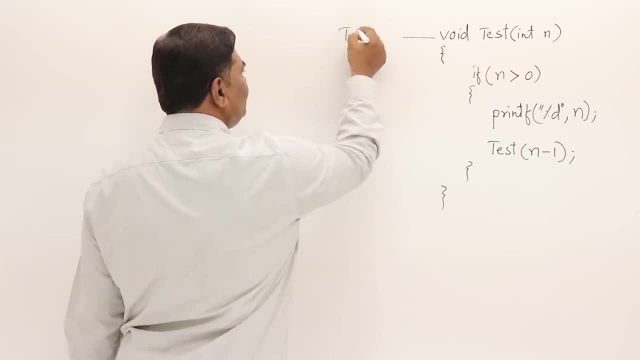 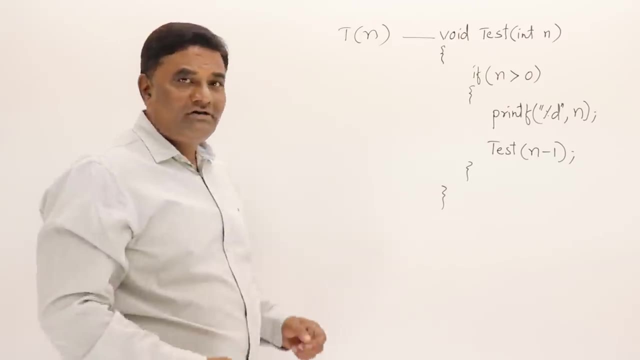 instead of f of n, I will call it as t of n. time taken by this algorithm is tn or this function is tn, Then that tn will be equal to what- The total amount of time taken by this one. So let us observe what is happening inside. Condition is checked. Let us ignore. 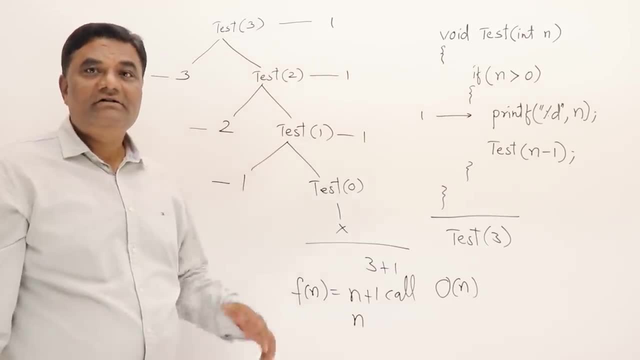 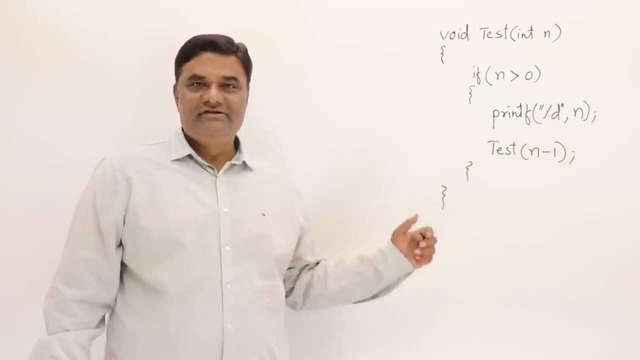 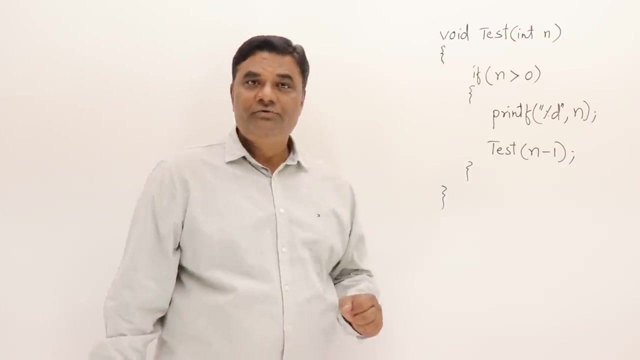 You can also call it as recursive tree or a tracing tree or a recursive tree I have used. Now let us find out how to prepare a recurrence relation for this function and how to solve that recurrence relation. Now, if any function or an algorithm is given to you, you can prepare. 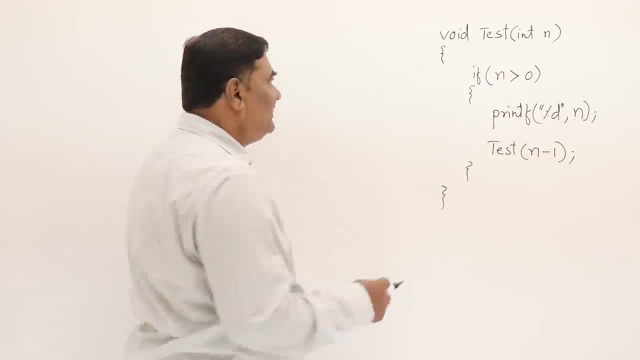 a recurrence relation as follows, Like this I am showing you. Assume that the time taken by this is f of n. No, Usually for recurrence relation, f of n is f of n times f of n times f of n. Function name is t, That is, t of n is used, So I will use the same thing. So instead of: 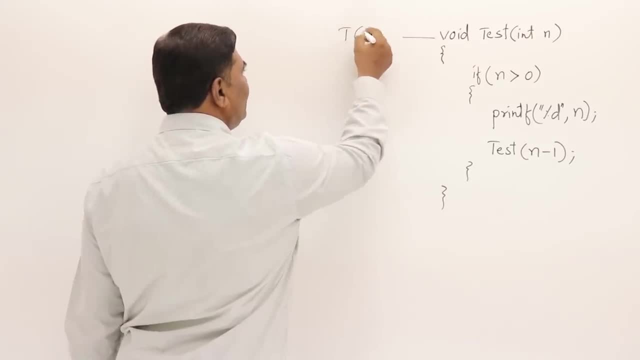 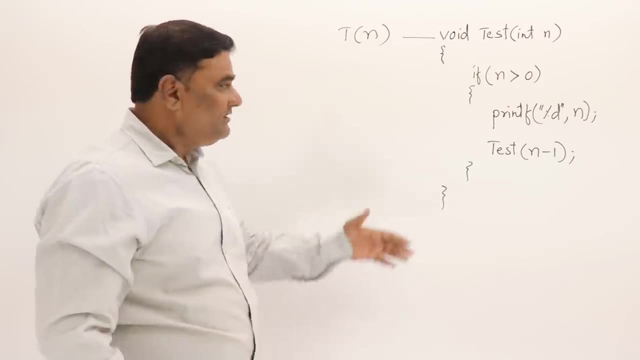 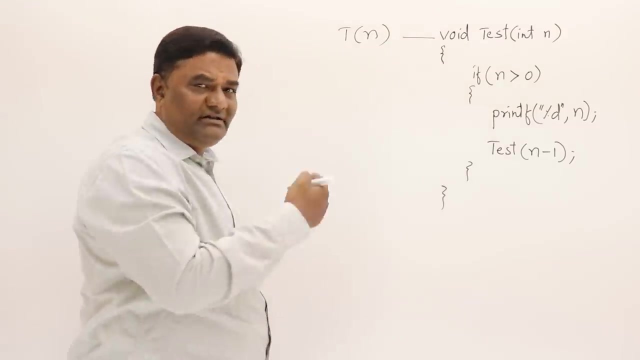 f of n. I will call it as t of n. Time taken by this algorithm is t n or this function is t n, Then that t n will be equal to what- The total amount of time taken by this one. So let us observe what is happening inside. Condition is checked. Let us ignore condition. 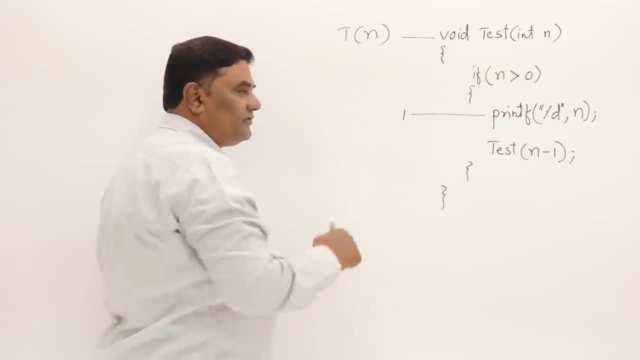 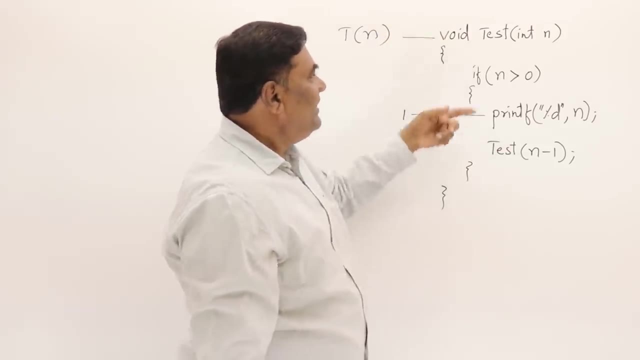 Inside that printf is there 1.. It will take 1 unit of time. The next, What is the next one? It is a recursive call. It is the same thing How much time we mention for this t n, Then what will be the time for this one t n minus 1.. Right, 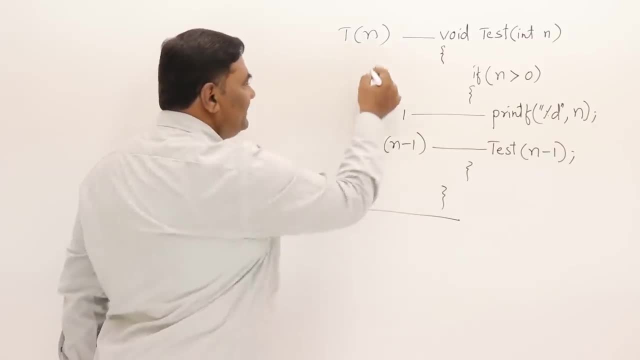 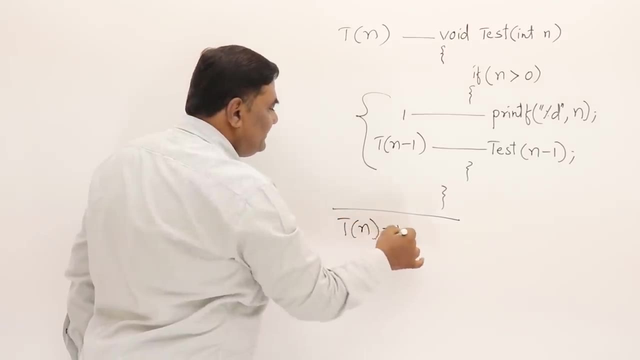 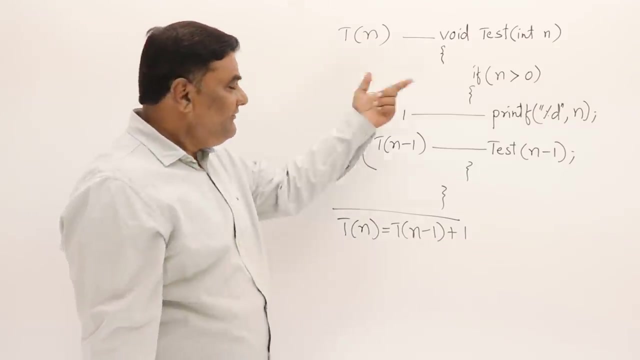 Now, that is it. So what is the total time, t n? I said that the total time taken by this part of an algorithm, So that t n is equal to t n minus 1 plus 1.. Now you can ask me why you have ignored condition. Say, if I consider: 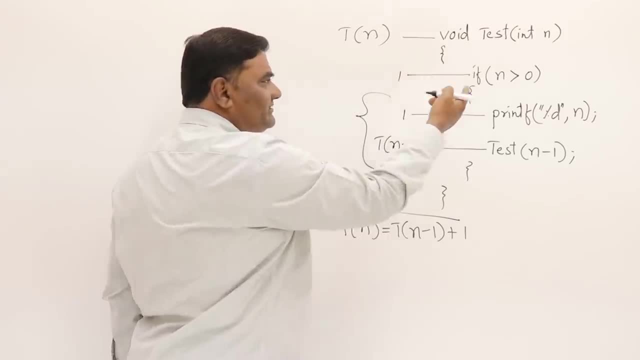 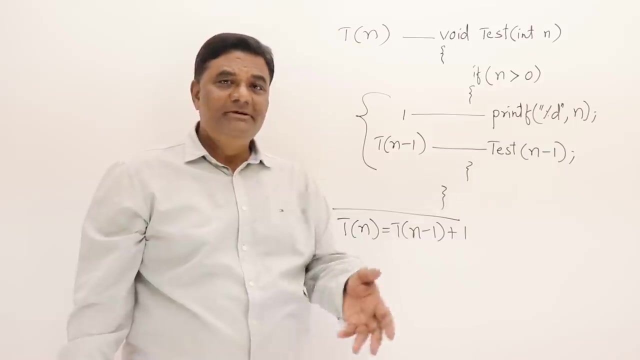 that condition also for one time, then it is just one condition. So one time. Then I will get 2 here. If I take 2 also, then the result of this expression will be same. only For the recurrence solution I will get the same answer. So if you have any constant value, you can simply make it. 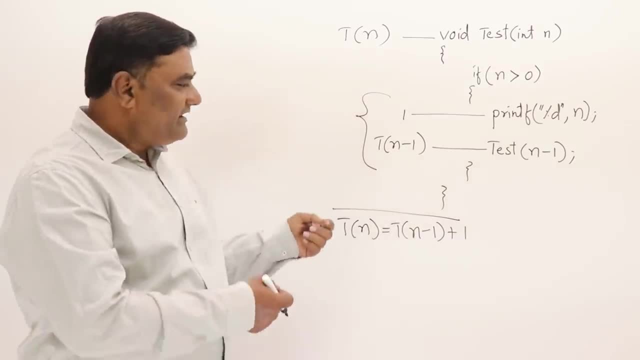 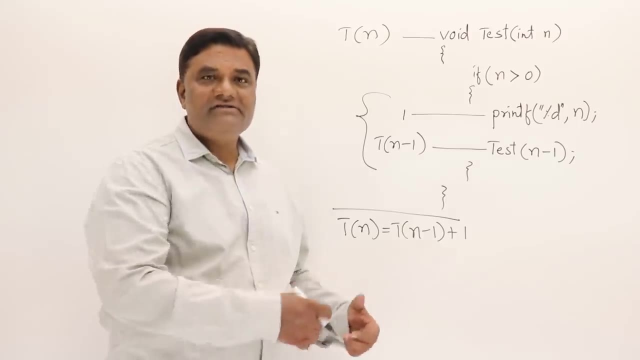 as 1 and use it. Or if you can write it as c also and use it constant, or some a as a constant, Some constant also, you can write and use it. So I prefer taking it as 1.. So if you have more than 1, then you can round it up to 1 only. Alright, This is the way. 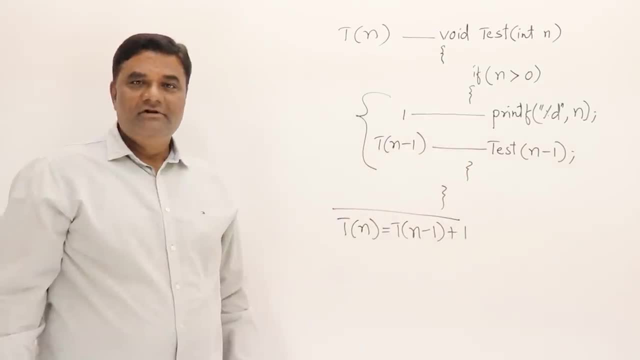 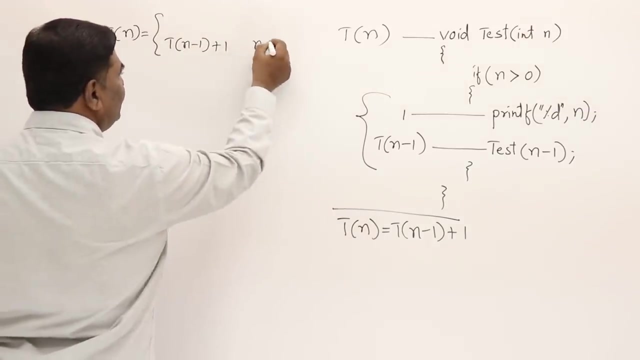 we write a recurrence relation. Now let us write a recurrence relation. So let us write a recurrence relation. So let us write a recurrence relation. t n is equal to t n minus 1 plus 1.. When n is greater than 0.. Yes, when n is greater than 0, this is the time. What happens if n is equals to? 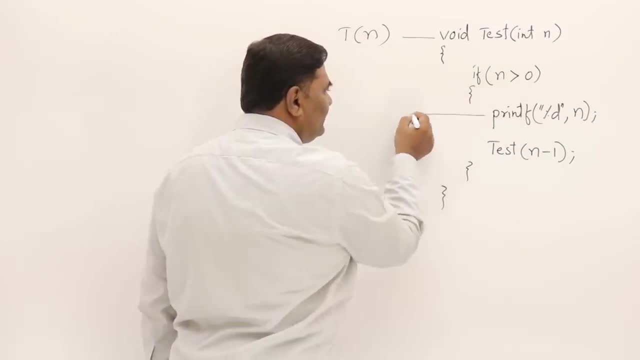 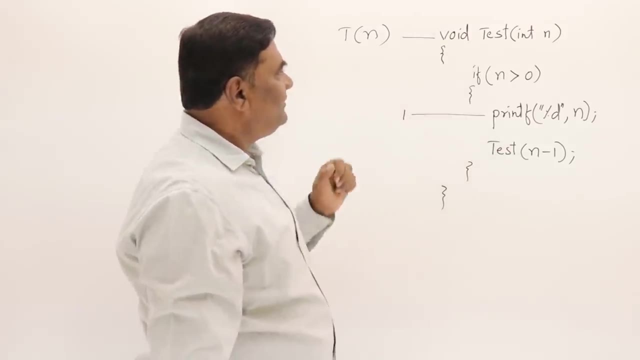 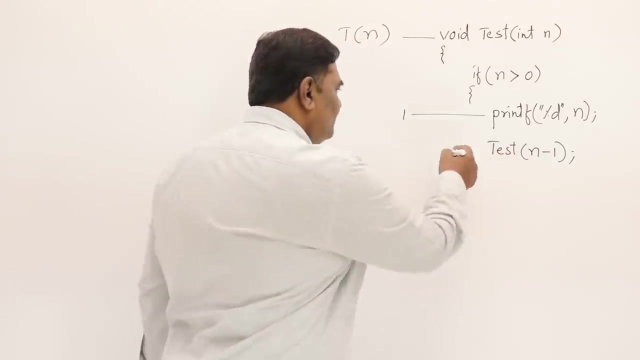 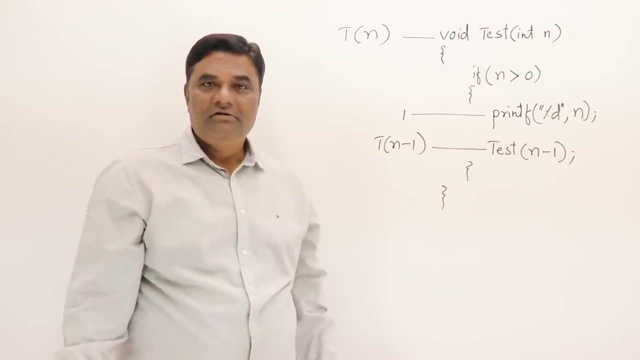 condition. Inside that printf is there One. it will take one unit of time. The next, what is the next one? It is a recursive call. It is the same thing How much time we mentioned for this tn, then what will be the time for this one? tn minus 1.. Right Now, that is. 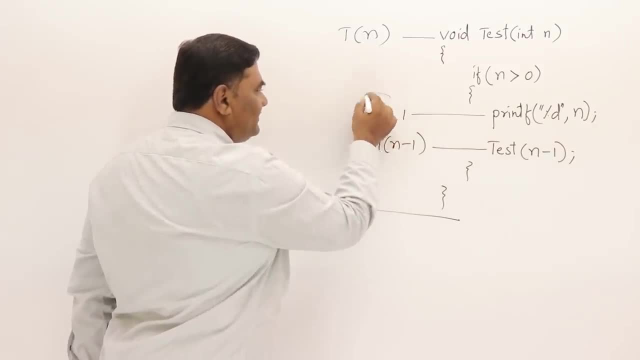 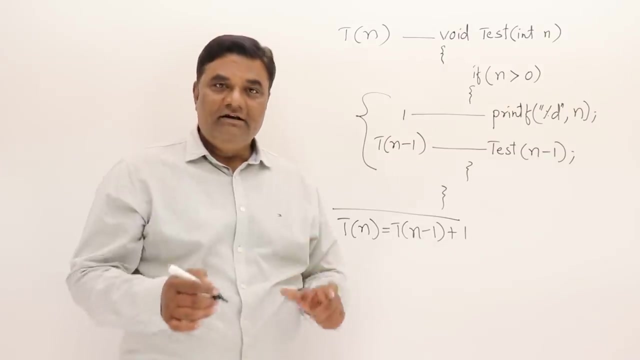 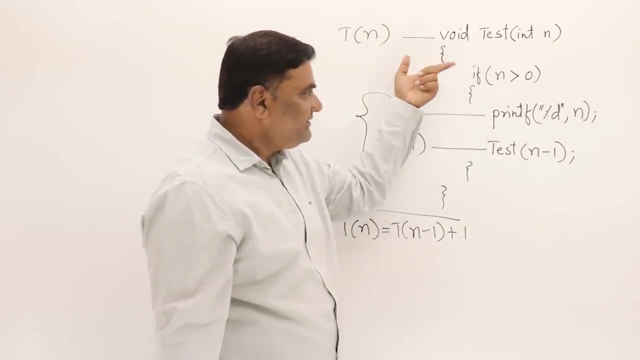 it. So what is the total time, tn? I said tn minus 1.. I said that the total time taken by this part of an algorithm, So that tn is equals to tn minus 1 plus 1.. Now you can ask me why you have ignored condition. Say if I consider that condition also for 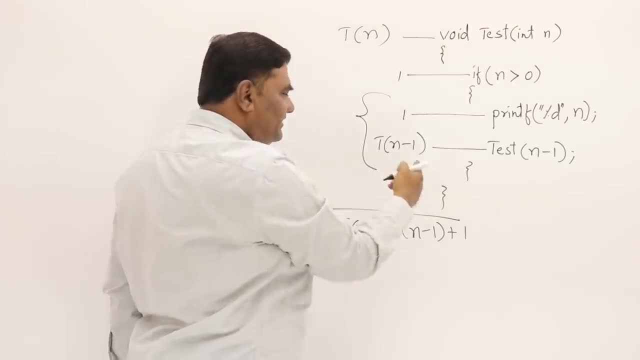 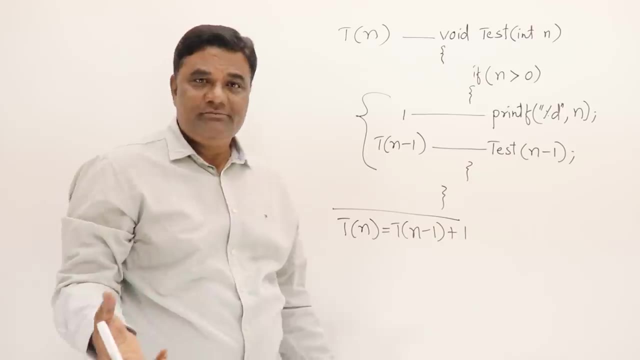 one time, then it is just one condition. So one time then I will get 2 here. If I take 2 also, then the result of this expression will be same. only For the recurrence solution I will get the same answer. So if you have any constant value, you can simply make it. 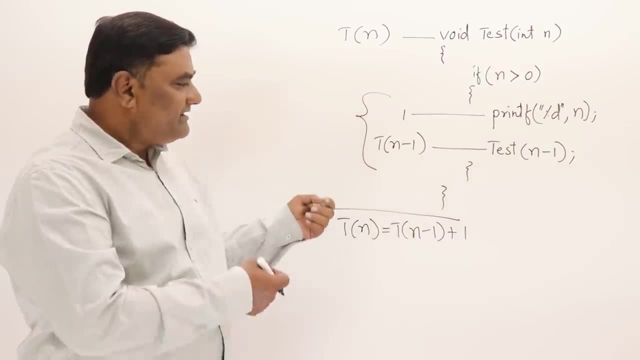 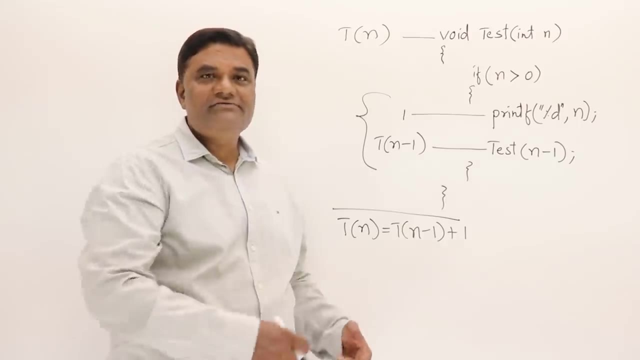 as 1 and use it. Or if you can write it as c also and use it constant, or some a as a constant, Some constant also, you can write and use it. So I prefer taking it as 1.. So if you have more than 1, then you can round it up to 1 only. All right, This is the way to do it. 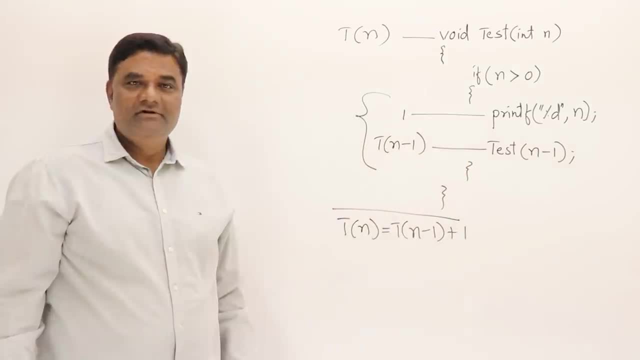 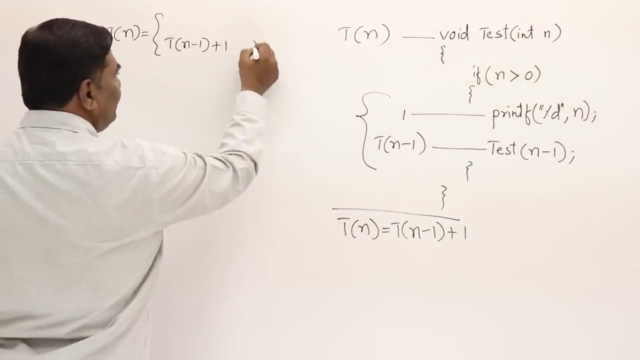 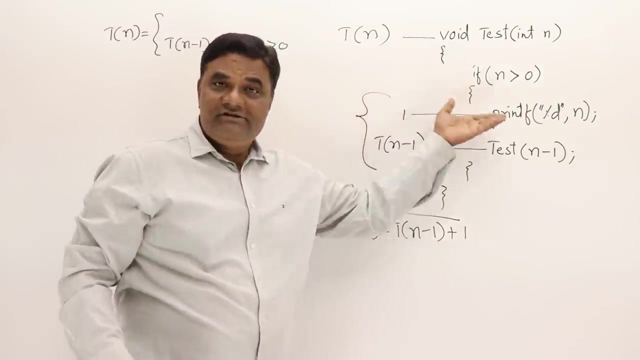 OK, Call recurrence relation. now let us write a recurrence relation. tn is equal to tn minus 1 plus 1.. When n is greater than 0., Yes. when n is greater than zero, this is the time. What happens if n is equals to 0? It is not doing anything if n is equal. to zero. So if n is equal to 0, it produces 0.. So let me just write the idea of recurrence relation. Tell me what it will be. Oh, over our analysis. it means t and n equal to 0.. Over our analysis. t and n. That is what we are doing. When n is greater than 0, we month n-1 plus 1.. those are two factors. So when t and n-1 are not equal, when n is greater than 0, but if a, then 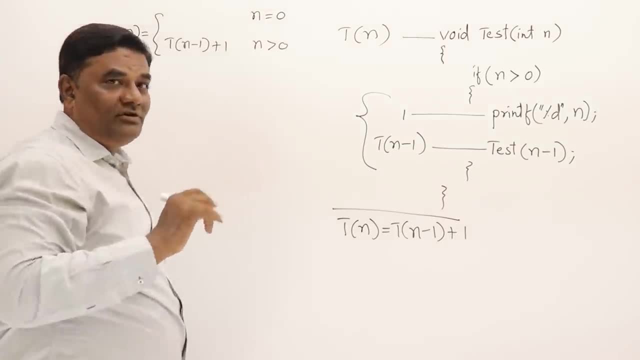 if 2 and t equals 1, then it equals two. this will mean t plus zero. Fore Know that if n equals 3, if 3 equals it, is not doing anything. so shall I write 0 here? no, the time we don't write it 0 if it is 0 also. 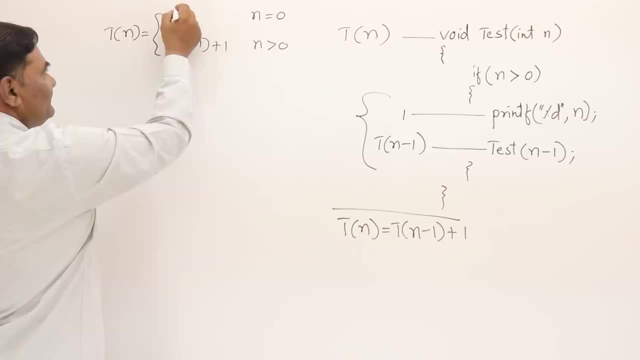 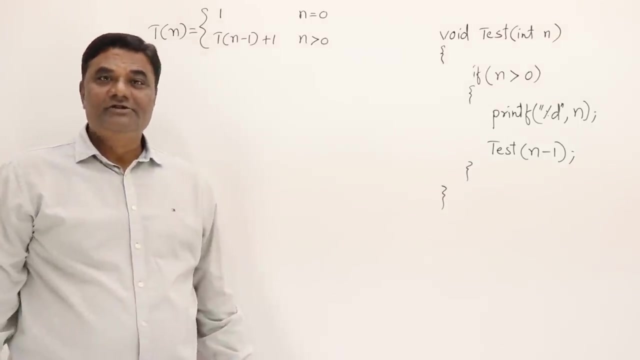 it's a constant, so we write it as 1. so I will take it as 1, or else you can make it as c or a or k, anything some constant you can write there. now let us solve this recurrence relation. now let us solve this recurrence relation by substitution method. back substitution, we will follow. let us take this: 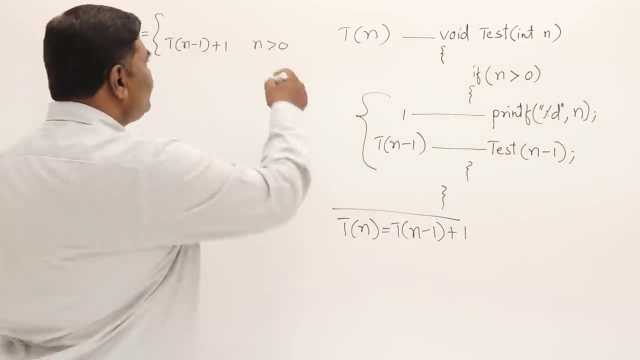 0?? It is not doing anything if n is equals to 0.. So if n is equals to 0, it is not doing anything. So shall I write 0 here? No, the time we don't write it as 0. We are not going. 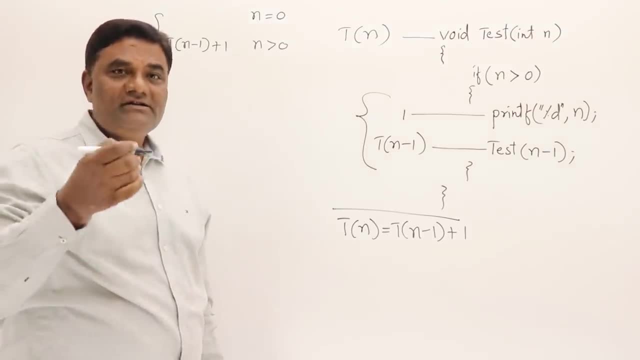 to write it as 0.. This time we do not write 0, we are going to write 0 when we don't write. If it is 0, also it's a constant, so we write it as 1.. So I will take it as 1.. 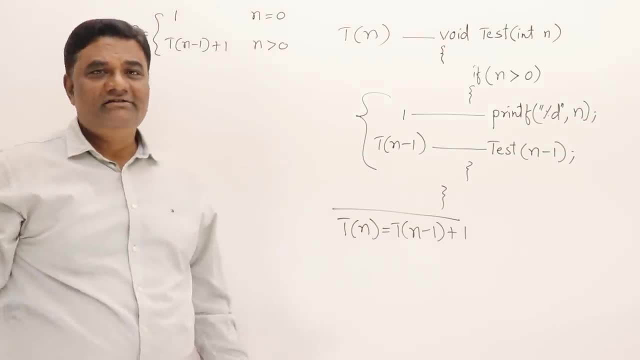 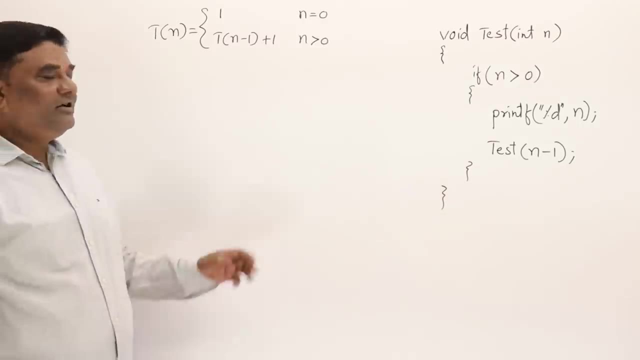 Or else you can make it as C or A or K, anything, some constant you can write there. Now let us solve this recurrence relation. Now let us solve this recurrence relation by substitution method. back substitution, we will follow. Let us take this. 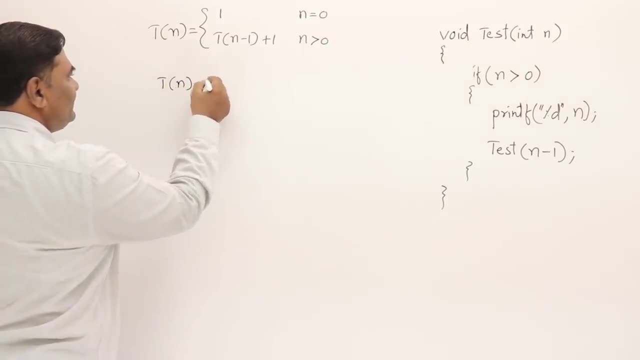 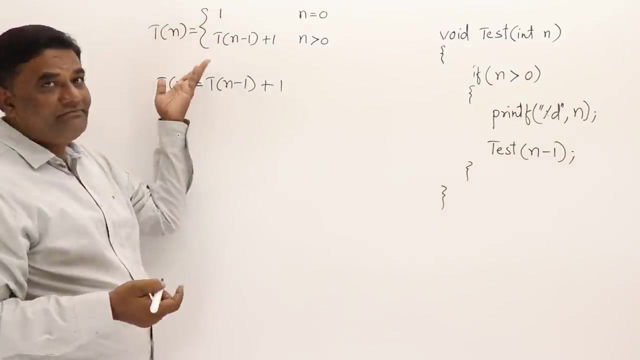 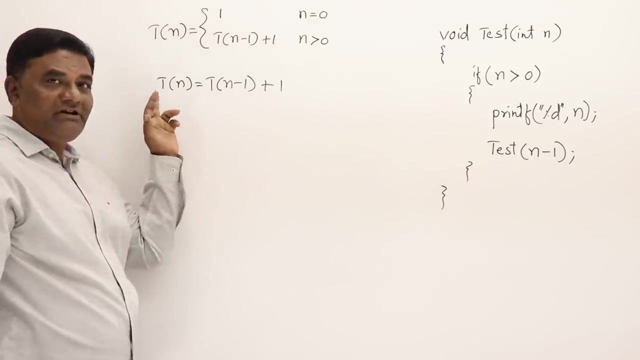 This is Tn is equals to Tn minus 1 plus 1.. We will solve this one. That is all that is solved. it is 1.. We have to solve this one. Now for solving this. I can know the answer for Tn if I know what is Tn minus 1.. 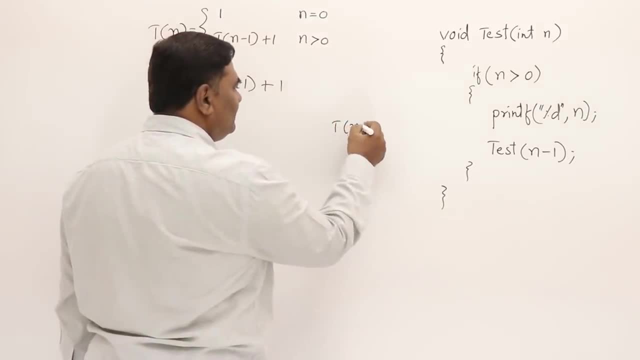 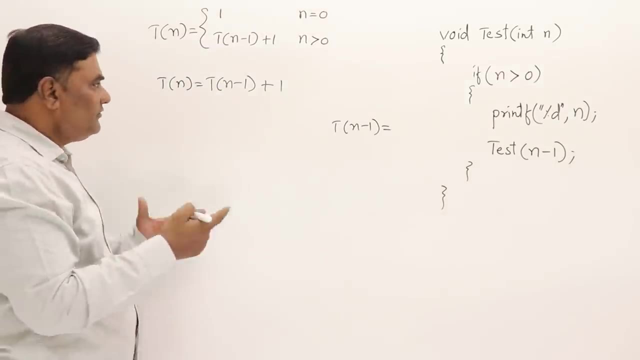 So what is Tn minus 1?? What is this? If I know, I will use it here. So I don't know: Tn minus 1.. But I know what is a Tn. Tn is equals to. 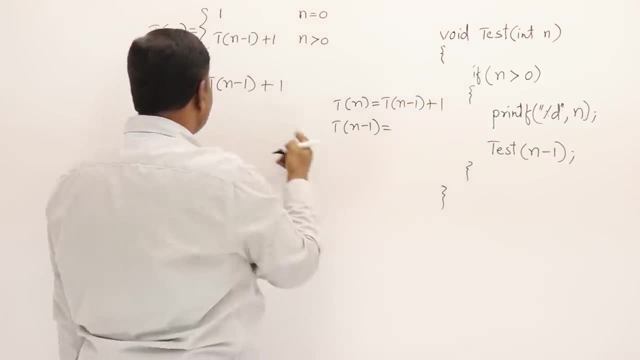 Tn minus 1 plus 1.. Yes, this is the 1. Then what will be Tn minus 1?? So if this is N and it is changed to N minus 1, so this is also N minus 1.. 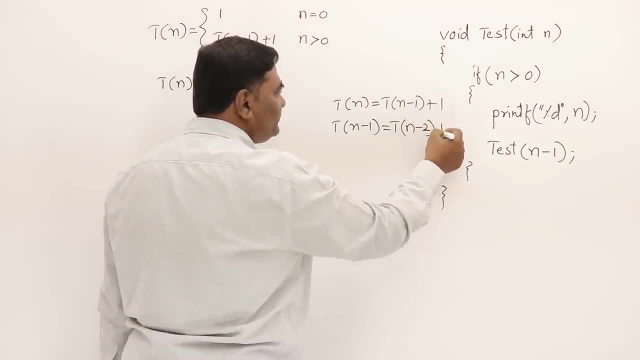 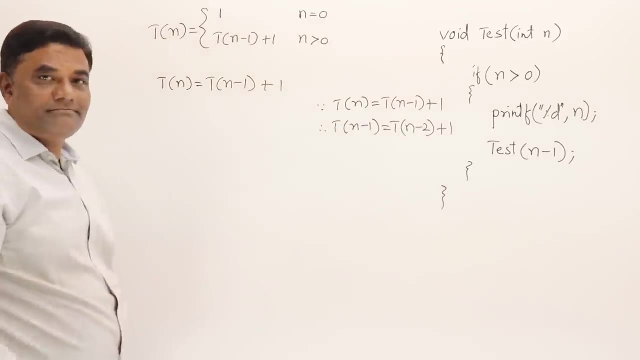 So this becomes N minus 1 minus 1, N minus 2 plus 1.. Okay, Since this is Tn, therefore Tn minus 1, is this one. Now substitute Tn. I'll write Tn minus 1 in this equation. 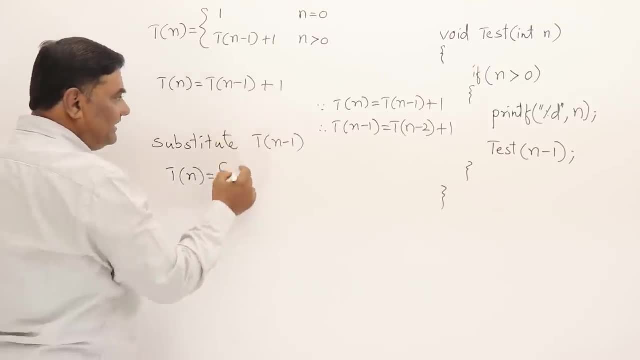 So Tn is equals to. in bracket I'll write this: Tn minus 1.. So what I got? Tn minus 2 plus 1 and plus 1.. So this part I have substituted here at this place. 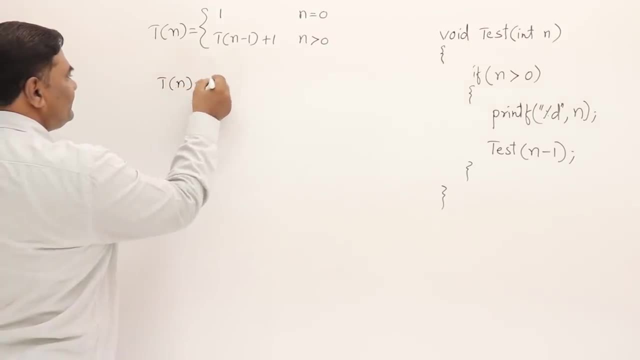 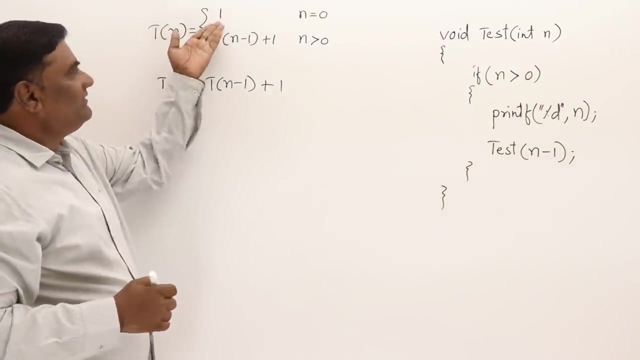 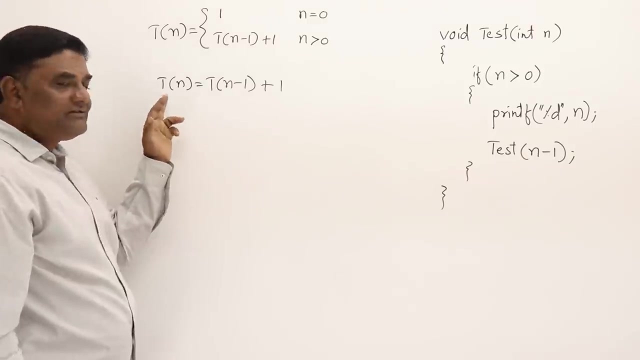 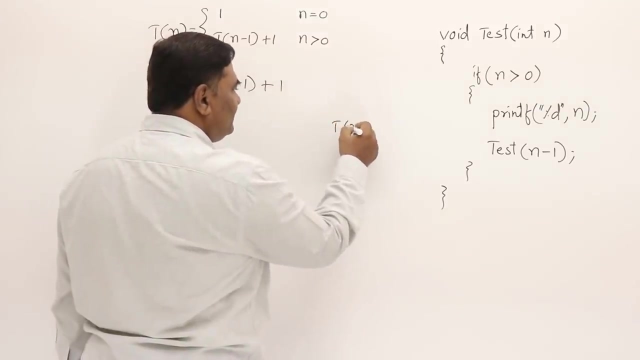 this is tn is equals to tn minus 1 plus 1. we will solve this one that is already solved. it is 1. we have to solve this one. now for solving this, I can know the answer for tn if I know what is tn minus 1. so what is tn minus 1? what is this? if I know, I will use it here. 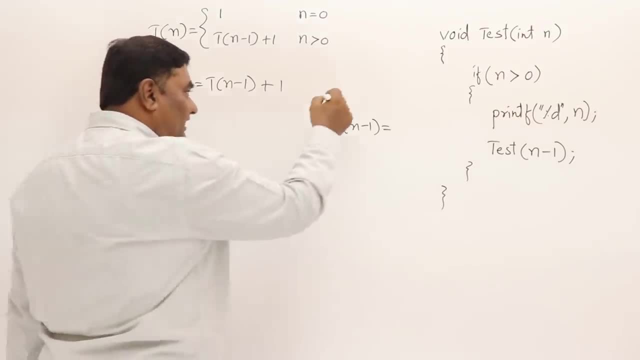 what is this? if I know, I will use it here. So I don't know tn minus 1, but I know what is a tn. tn is equals to tn minus 1 plus 1. yes, this is the one. then what will be tn minus 1.. So if this is n and it is changed to n, 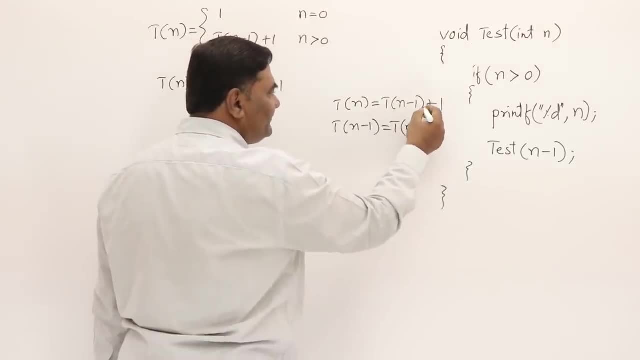 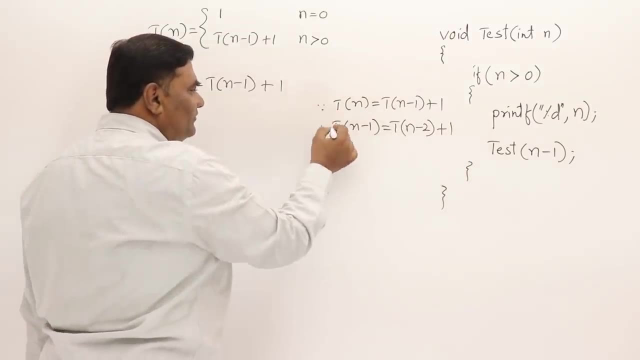 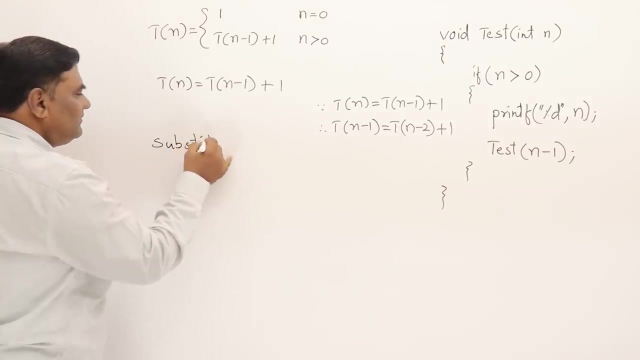 minus 1, so this also n minus 1, so this becomes n minus 1 minus 1, n minus 2 plus 1. okay, Since this is tn, therefore tn minus 1, is this one Now substitute tn minus 1 in this equation. 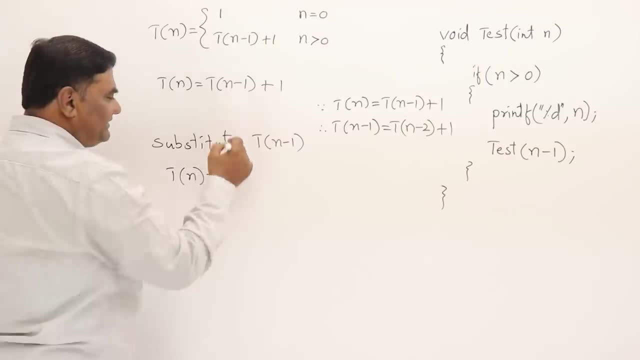 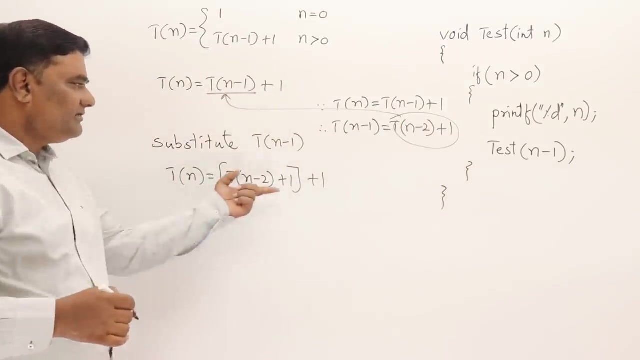 So tn is equals to. in bracket I will write this: tn minus 1. so what I got? tn minus 2 plus 1 and plus 1.. So this part I have substituted here 1. At this place. so I got this one. 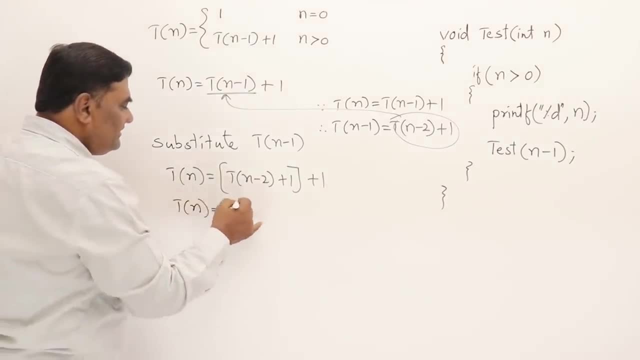 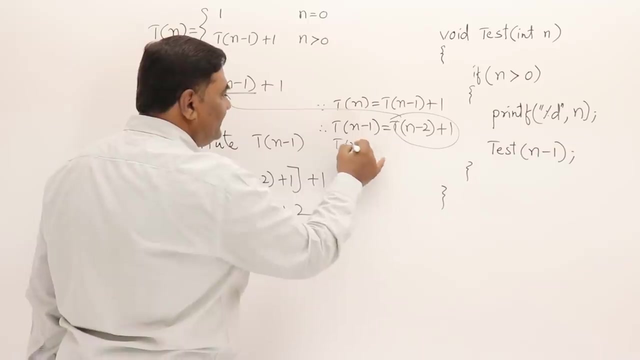 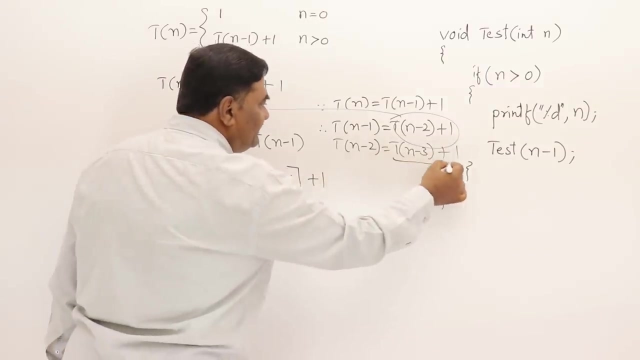 Then this is: tn is equals to tn minus 2 plus 2. 1 plus 1, 2. If I substitute again, then tn is equals to what will be tn minus 2, tn minus 3 plus 1.. See this, tn minus 2 will be equal to tn minus 3 plus 1. yes, I have substituted this portion here. 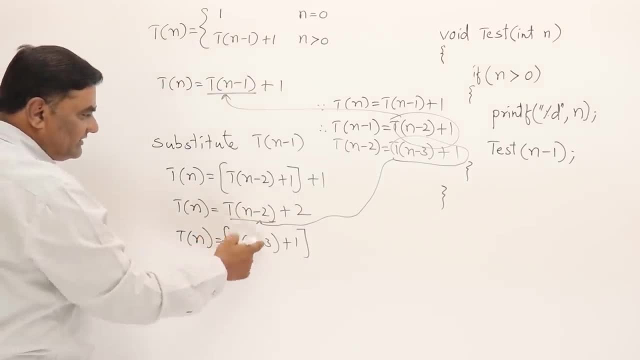 right at this place. So I have written this. then plus 2 is as it is Now. if I solve this one again, then tn is equals to tn minus 3 plus 3. that's what I got. So how many times I am going to do this? 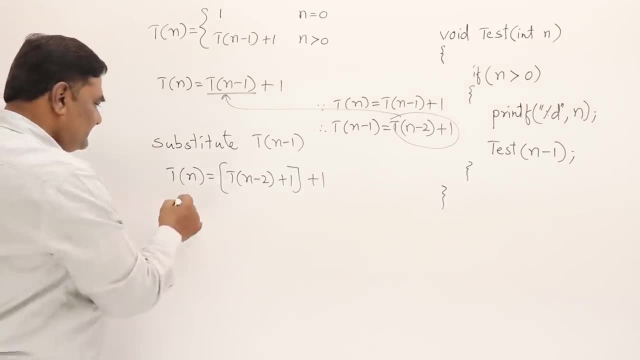 So I got this one. Then this is: Tn is equals to Tn minus 2 plus 2, 1 plus 1, 2.. If I substitute again, then Tn is equals to what will be Tn minus. 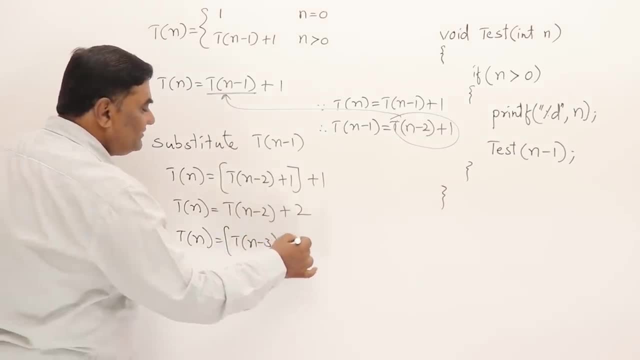 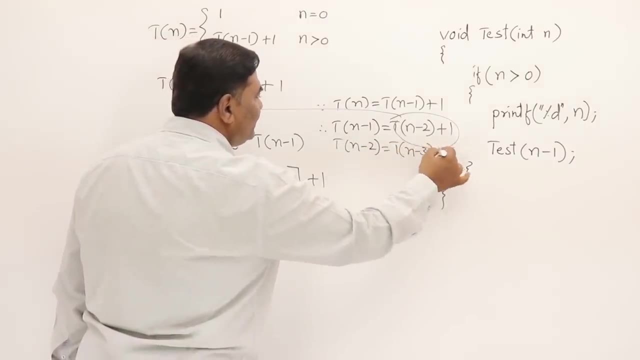 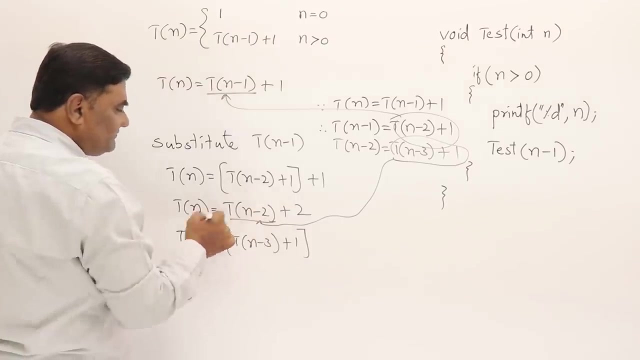 2? Tn minus 3 plus 1.. See this: Tn minus 2 will be equal to Tn minus 3 plus 1.. Yes, I have substituted this portion here right at this place, So I have written this Then: 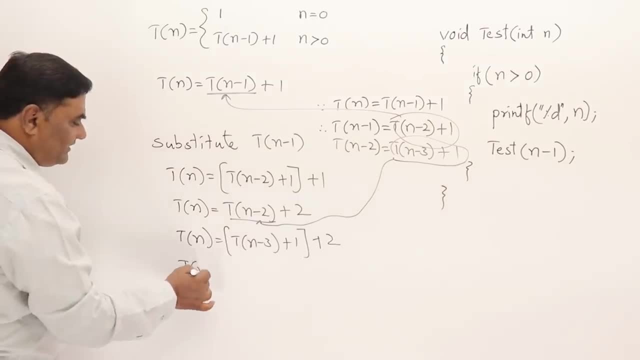 plus 2 is as it is Now. if I solve this one again, then Tn is equals to Tn minus 3 plus 3.. That's what I got. So how many times I should do this? See when I got 2 times that. 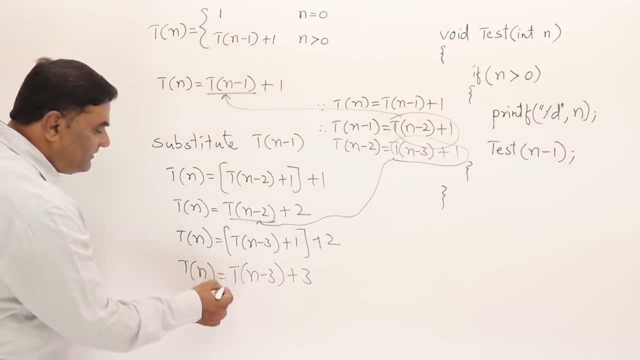 is sufficient. You can continue further And I say that I am going to continue this. How long For k times? Continue for k times. If I continue for k times, what I get, See if you observe when I did for one time it. 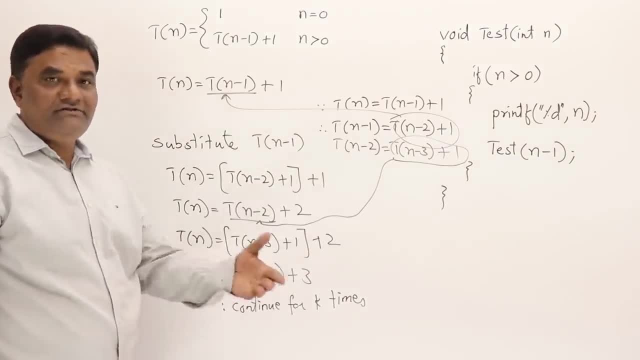 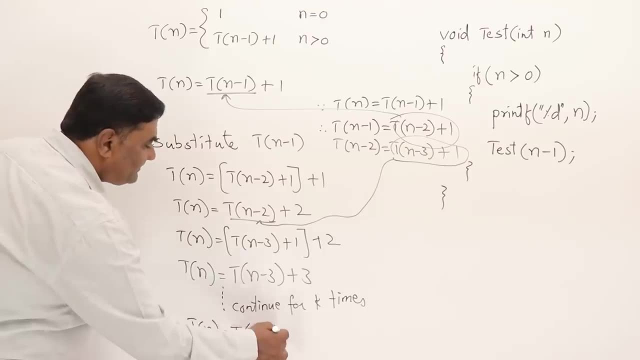 was 2,, next time it was 3,, then it goes on, so it will be k, So this will be: Tn is equals to Tn minus 3.. Yes, n minus k plus k. So this is the important one for me. now I will continue here. What? 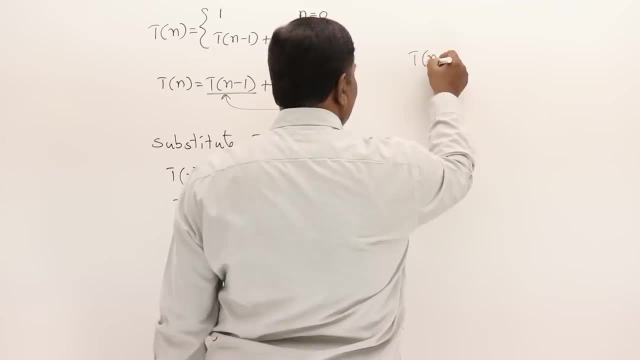 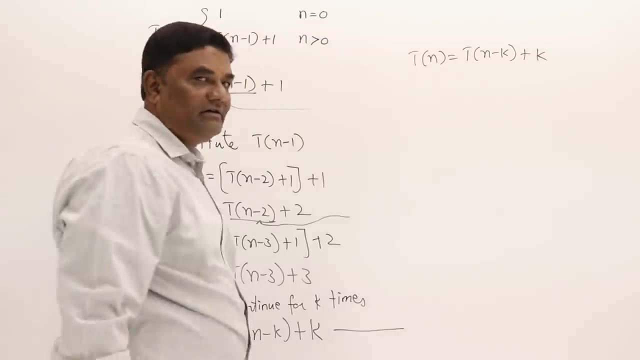 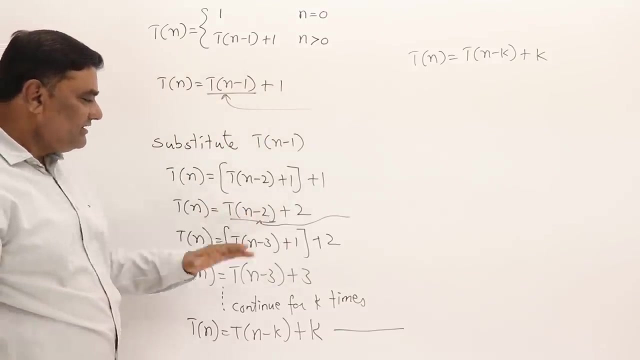 is the equation I got: Tn is equals to Tn minus k plus k. See, it was Tn minus 1 plus 1. Substitute it: I got Tn minus 2 plus 2.. Substitute it: I got Tn minus 3 plus 3.. Continued. 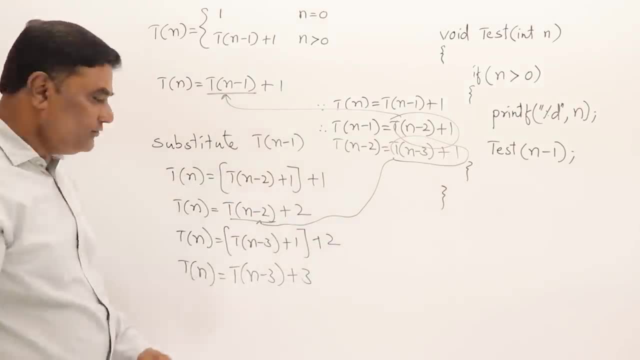 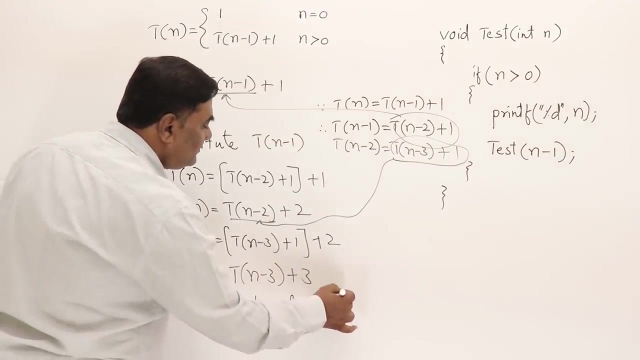 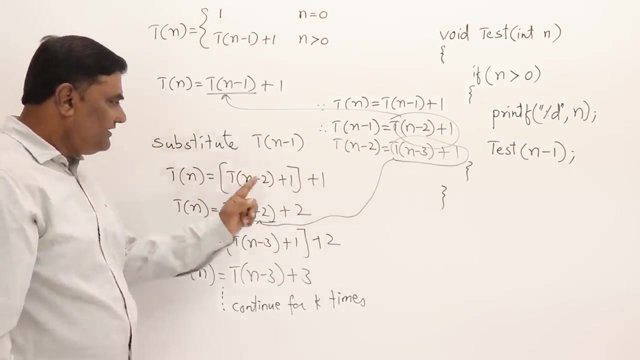 See when I got 2 times. that is sufficient. you can continue further and I say that I am going to continue this. how long for k times? continue for k times. If I continue for k times, what I get. see, if you observe when I did for 1 time, it was 2. 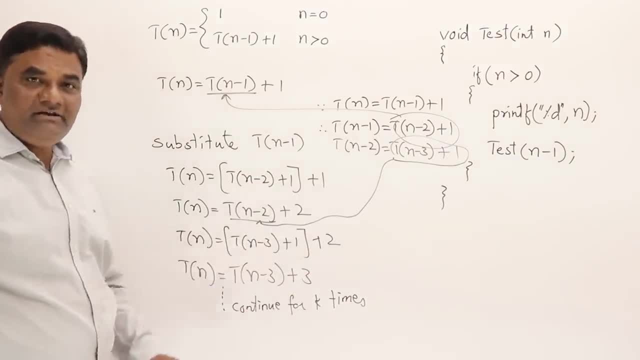 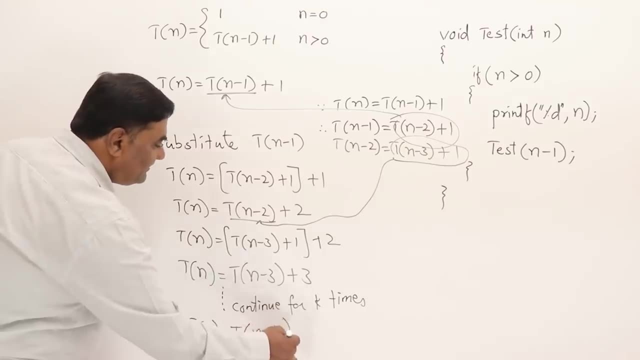 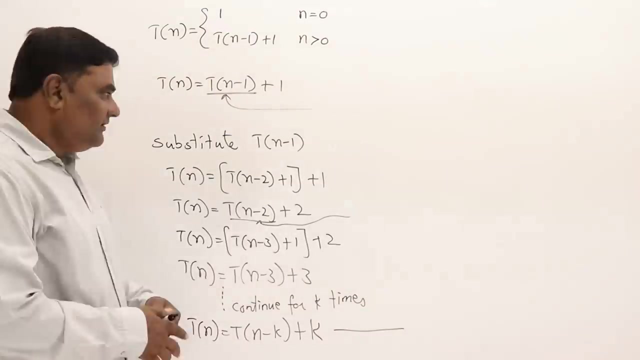 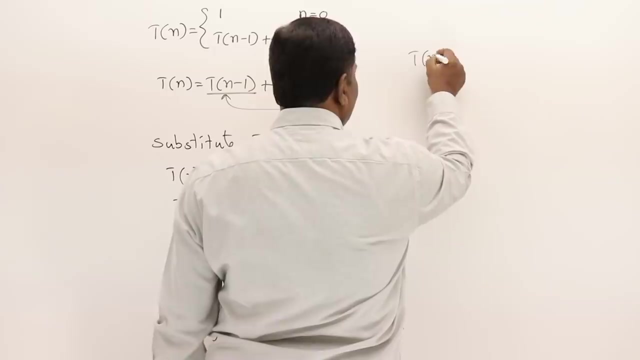 next time it was 3.. Then it goes on, So it will be k. so this will be: tn is equals to tn minus k plus k. So this is the important one for me. now I will continue here. What is the equation I got? tn is equals to tn minus k plus k. 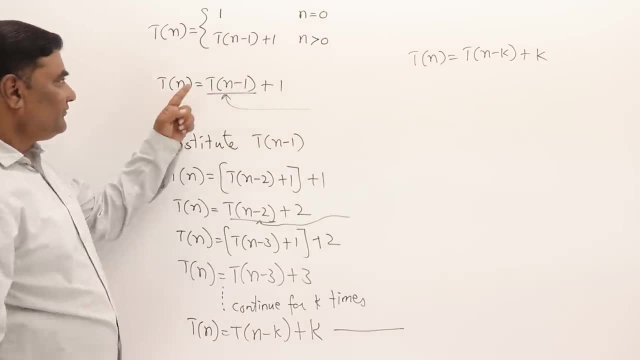 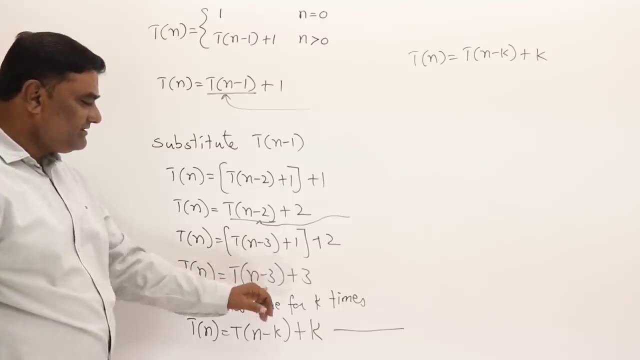 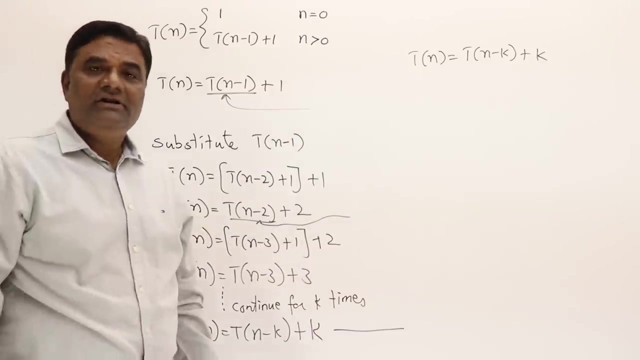 See. See, It was tn minus 1 plus 1. Substitute it. I got tn minus 2 plus 2.. Substitute it, I got tn minus 3 plus 3, continued up to k. so tn minus k plus k this one. So I said that I will stop at k. 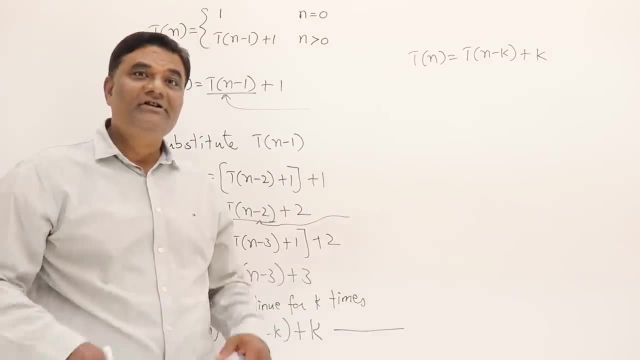 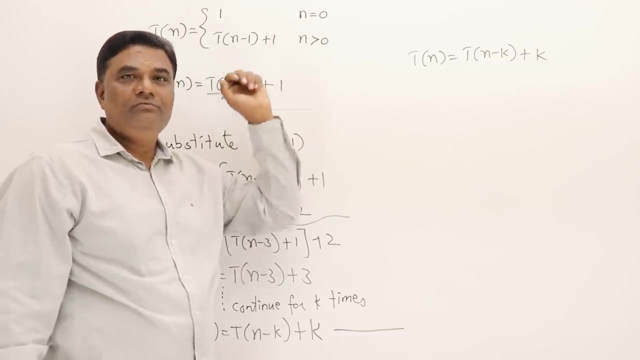 k means some steps after some steps. I will stop after k steps, k substitutions. I will stop Now. What is the smaller value? I know What is the smaller value. I know I know n is equals to 0. if n is equals to 0, I know it is 1, answer is 1.. 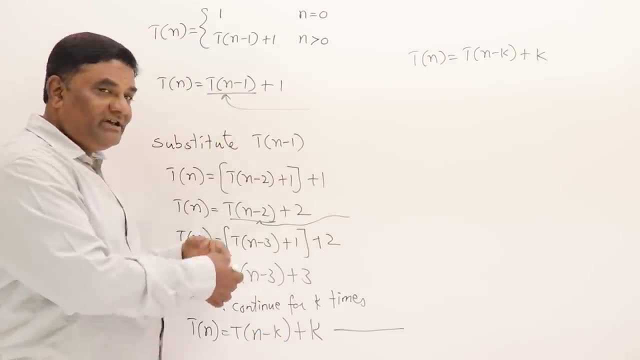 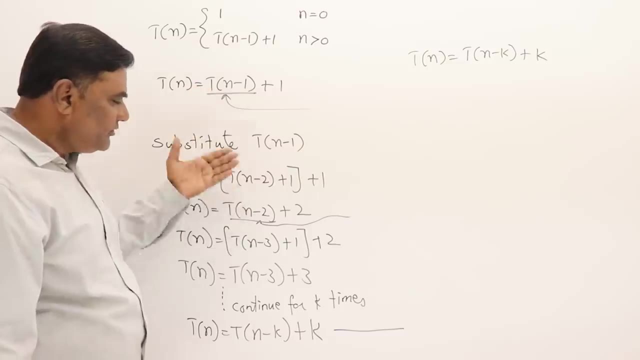 So here, n minus 1, was there? so minus 2, then 3, then 4. if you go on subtracting like this, at one point it should become 0. So the my purpose was to go on substitute and reach till n equal to 0. 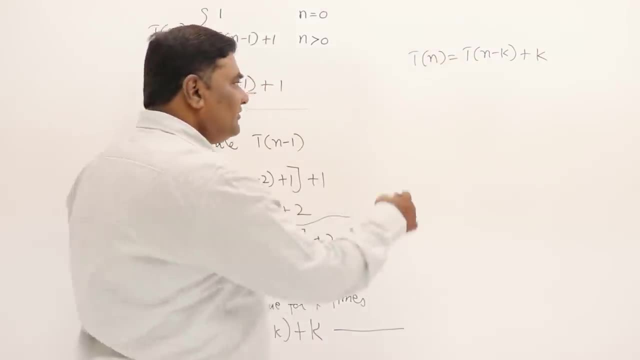 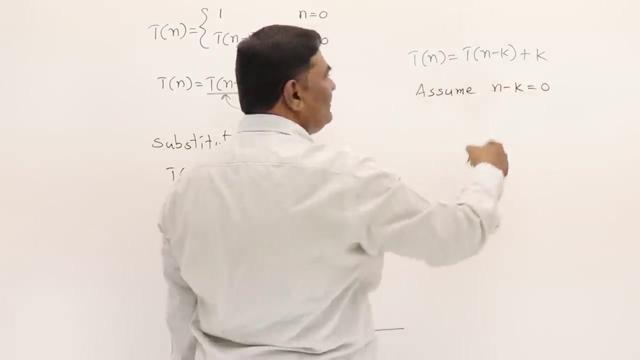 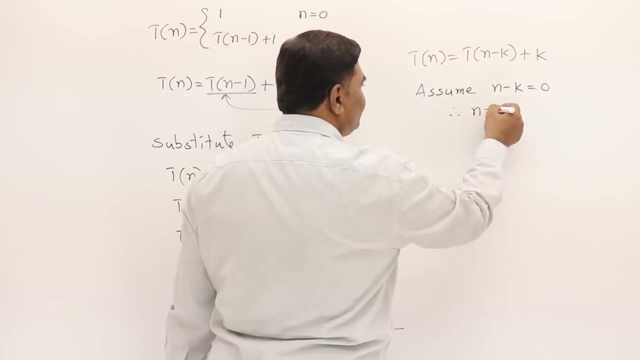 So I assume that I have reached at 0.. So I assume this: 0.. n minus k is 0. I will assume this means I have reached till there. when I say n is minus k is equals to 0. therefore n is equals to k. 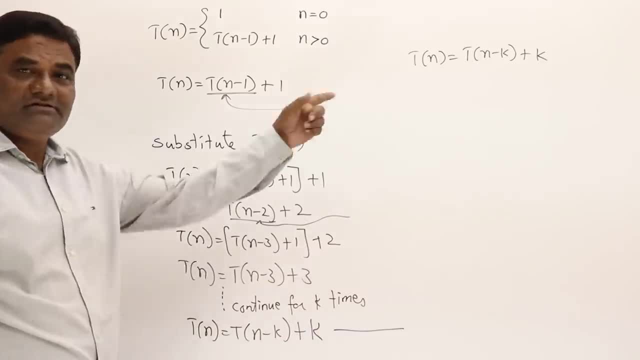 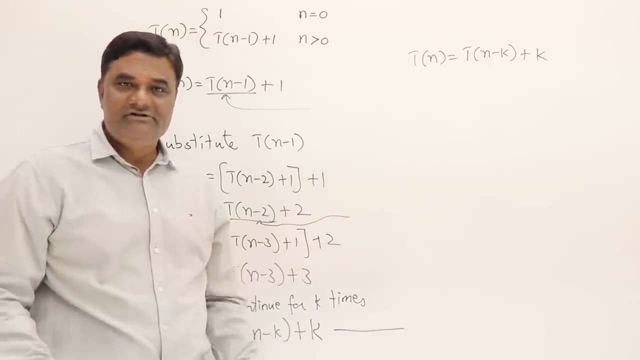 up to k. So Tn minus k plus k. So I said that I will stop at k. k means some steps After some steps. I will stop After k steps, k substitutions, I will stop Now. what is the smaller value? I know, I know n is equals to 0.. 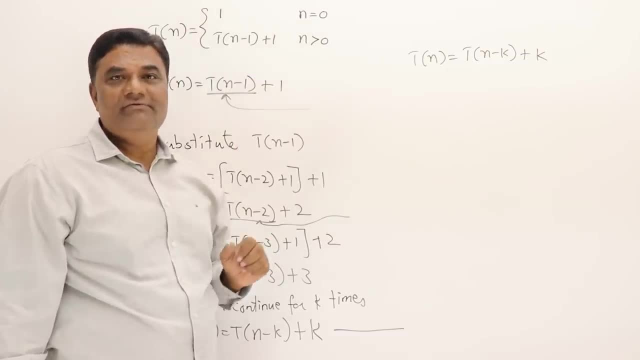 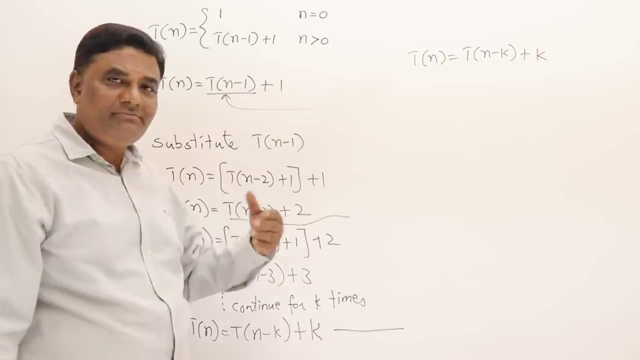 If n is equals to 0,, I know it is 1.. Answer is 1.. So here, n minus 1, was there? So minus 2, then 3, then 4.. If you go on subtracting like this, at one point it should become 0. 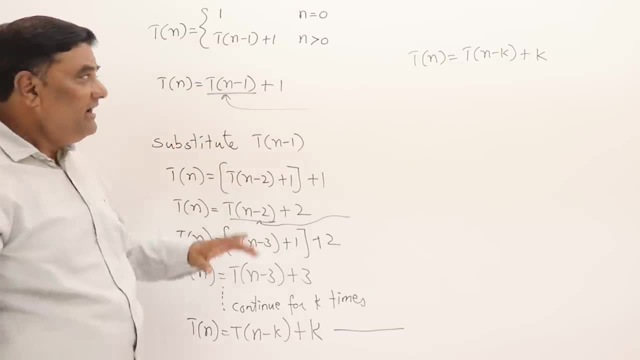 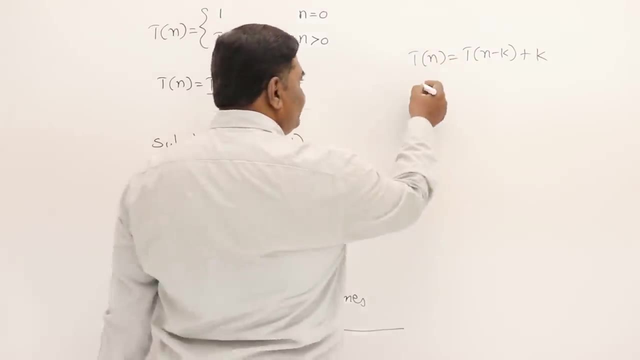 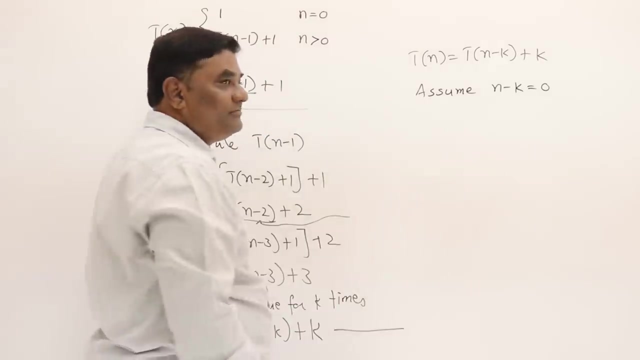 So my purpose was to go on substitute and reach till n equal to 0. So I assume that I have reached at 0.. So I assume this n minus k is 0. I will assume this Means I have reached till there. When I say n minus k is equal to 0,. 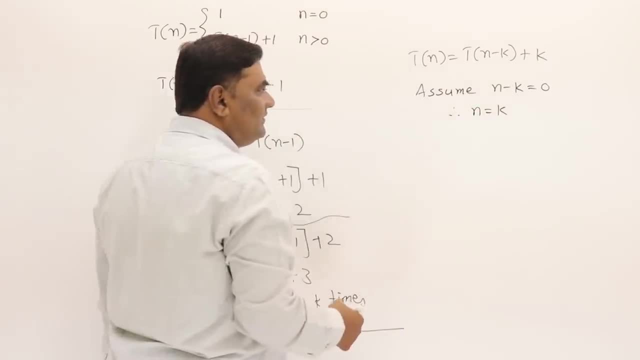 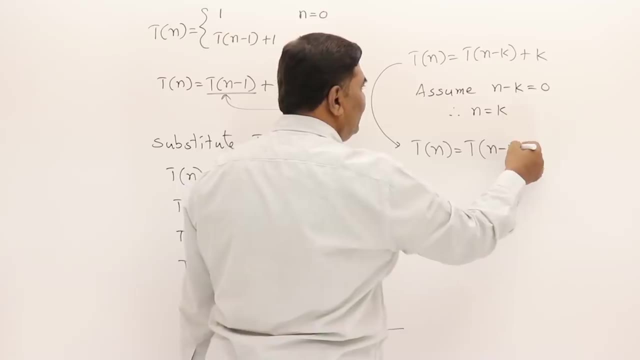 therefore, n is equals to k, Then what this will be, This will be: Tn is equals to Tn minus n plus n. Then Tn is equals to what is this T0 plus n? So this is what is a T0? T0, we. 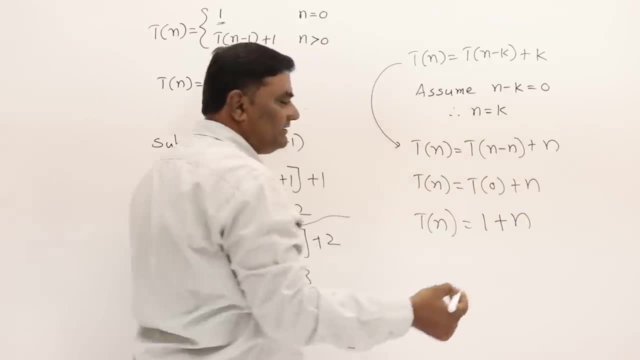 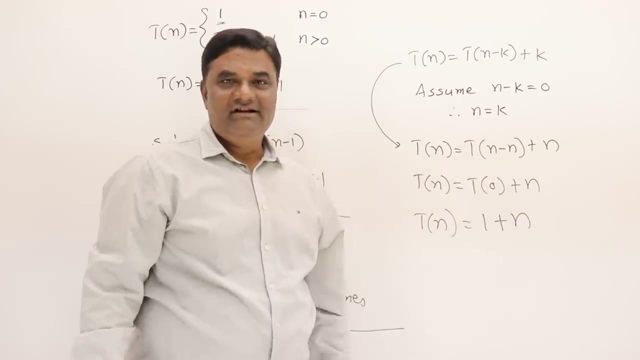 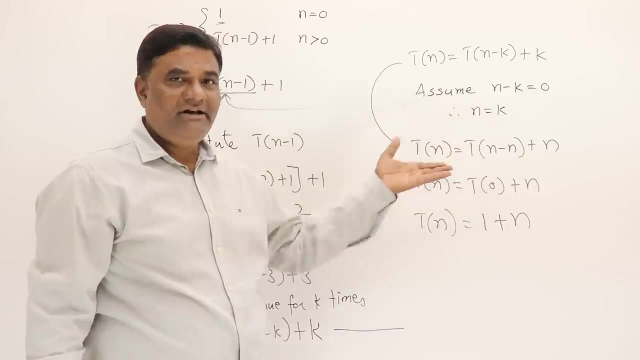 already know it. It is 1 plus n. That's it, It is solved. What the answer I got. you see, 1 plus n is the time. So just now I have shown you how we can prepare a recursive tree and find the time for that algorithm. Actually, I made a tracing, as well as along with that. 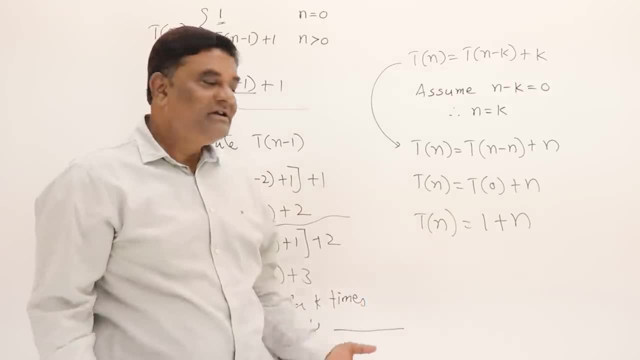 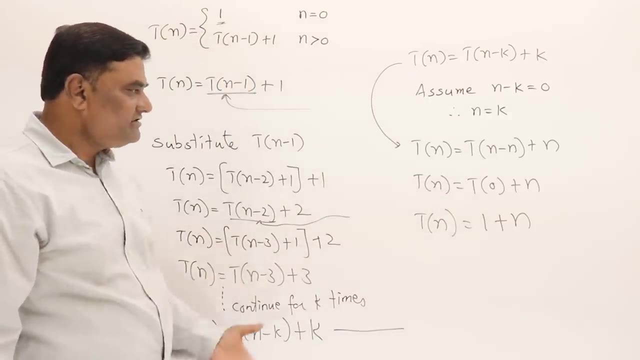 recursive tree. So there also I got n plus 1 calls. Here also I am getting the answer as n plus 1.. So I have prepared a recurrence relation, solved that problem, solved that problem, recurrence relation, and i got this answer. and this is again order of n. see, actually this belongs to. 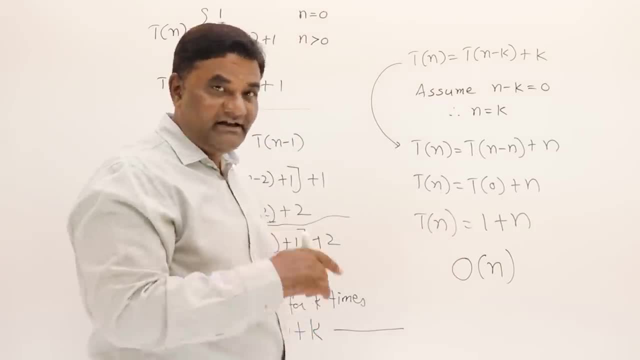 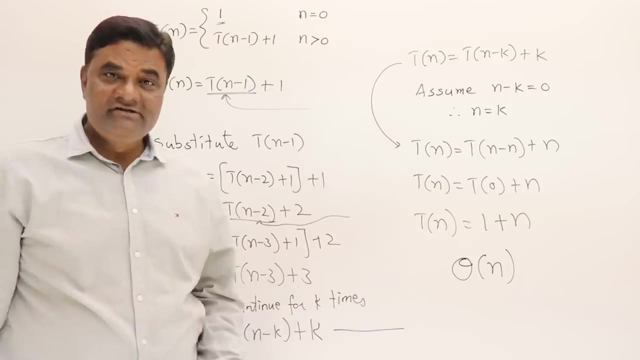 a class, linear class order of n, that is n, so i can call it as theta of n. that's it. this is the first recurrence relation. so i will show you more and more recurrence relation. so i will take the program, i will prepare the recurrence relation and i will solve it. so continue watching rest. of the videos.